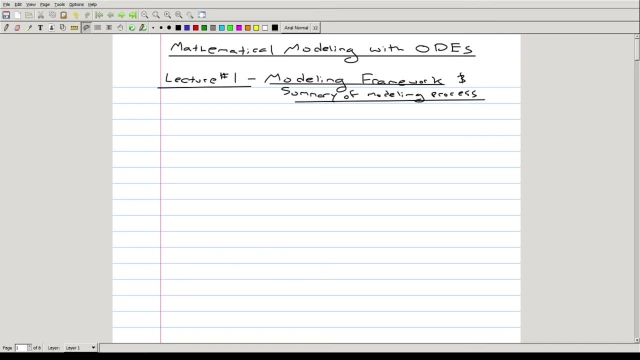 Hello everyone and welcome to today's lecture. Today I'd like to start off by answering a question which is the main question dealing with what we'll be talking about in this course, and that is: what is a mathematical model? And this is going to be the main thing that we'll be studying in this course. So before we get started, we want to kind of have a good idea of exactly what a model is and what it constitutes. 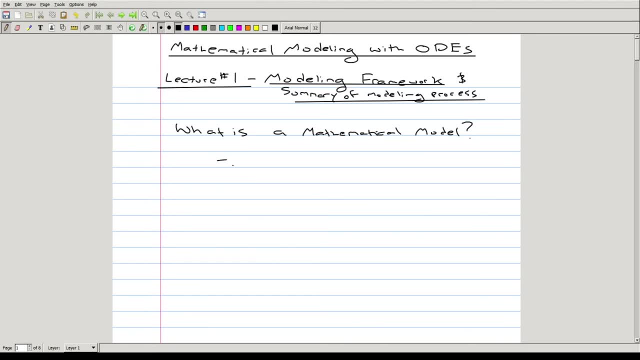 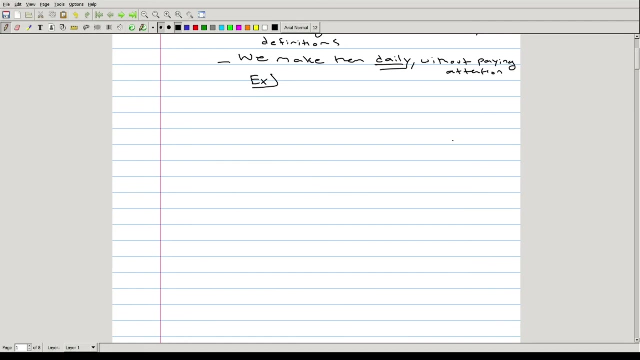 I guess I should start off by saying that this is a loaded question with many possible definitions. We make mathematical models daily without even thinking about it or without paying attention. And to give you a good example of this, think about. one of the most basic questions that you might ask yourself is: how do I get downtown or how do I get to a place? 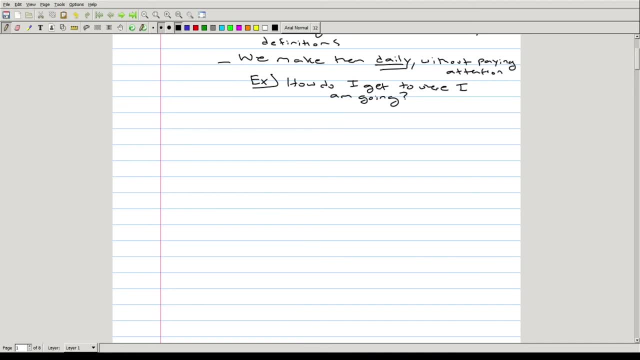 And there's many factors that you might consider, and you might not even realize that you're considering and weighing these factors against one another, But for one, the distance of where you're going is one of the factors that is going to factor into this decision. 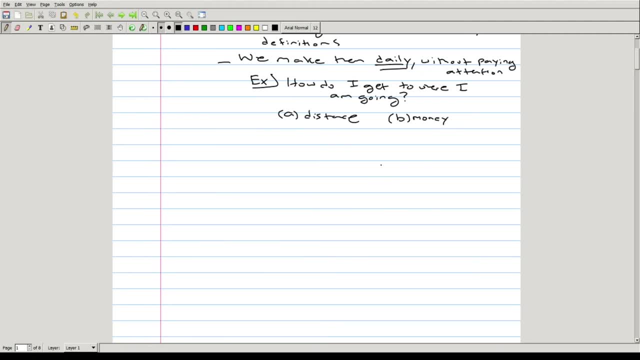 The money that you want to pay to get there, Whether you want to take the bus or ride a bike or drive a car. And this brings up another very important factor, which is time, Or traversal time. How long do you want to take on the trip? 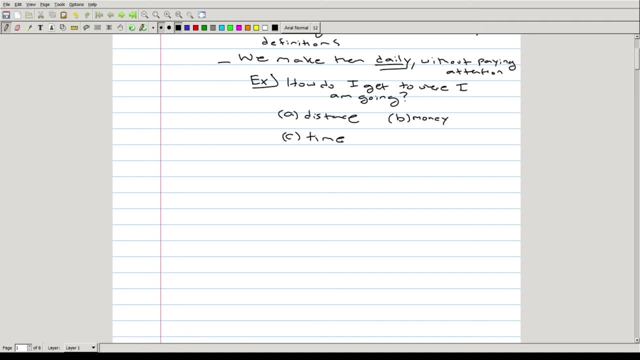 Do you want to walk, Take a very long time, but if it's a short distance, you can walk in no time at all. Another consideration that you might make is security. How do you want to get there? Are you bringing money with you? Are you carrying money on you or anything valuable on you? 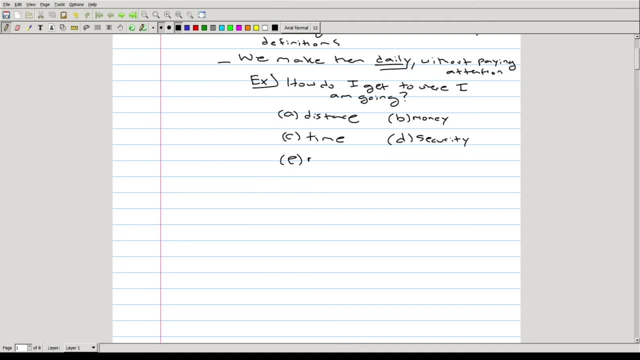 And then this also brings up- you know, all these are kind of related to one another- but the means of transportation. So are you taking the bus, Are you going to order an Uber? Are you going to bike? No, Another factor is: you know your mood. 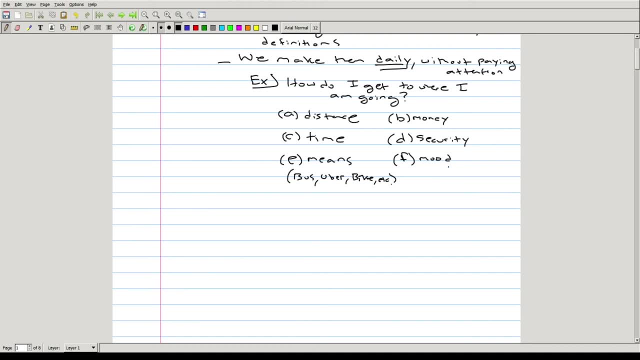 Are you rushing? It's kind of related to time and distance. Are you rushing to get somewhere? Are you having a kind of a leisurely stroll? But you know, there are many other examples and there are also, in this example, many other factors that you might want to consider. 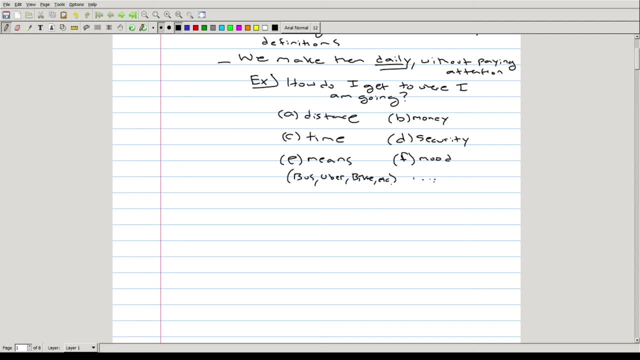 But here's one simple example of how we create a mathematical model. you know all the time When we're solving problems without even realizing it sometimes. So to put a definition down to mathematical modeling is not necessarily the easiest goal, but again, like I said, I'll try to describe it. 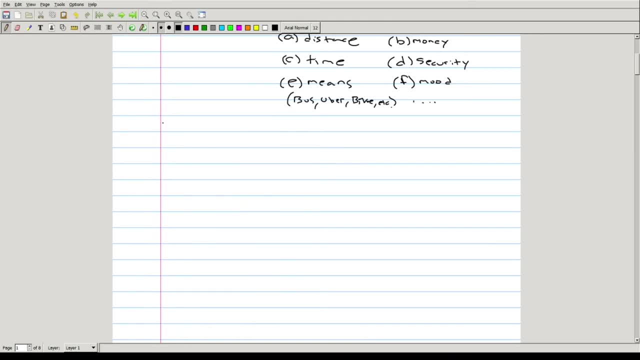 And a lot of the examples and the material. specifically, this definition that I'm about to write down comes from a very, very, very good textbook from one of my advisors, Meier-Humey, And this is the textbook Introduction to Mathematical Modeling. 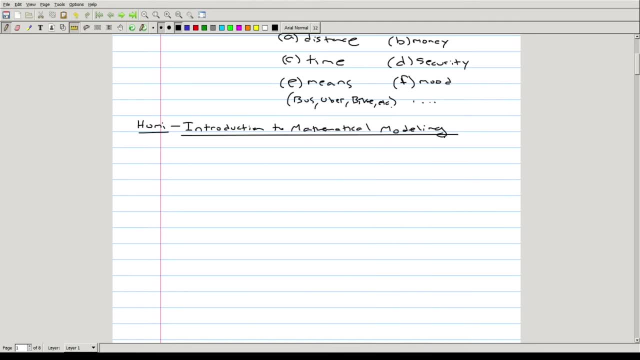 And if you're going to get any companion textbook for this course, I would recommend this textbook in addition to the others that I've provided in the syllabus, because this is a fantastic, fantastic overview and in-depth look at many of the modern aspects to mathematical modeling. 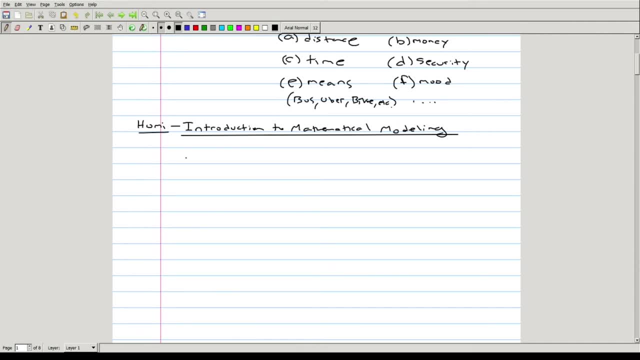 But right now I'll write down the definition to mathematical modeling given in his book. In general, modeling is the art of describing things in symbolic language. This is where your mathematical and physics theories come in. This is where you know organic verändert. 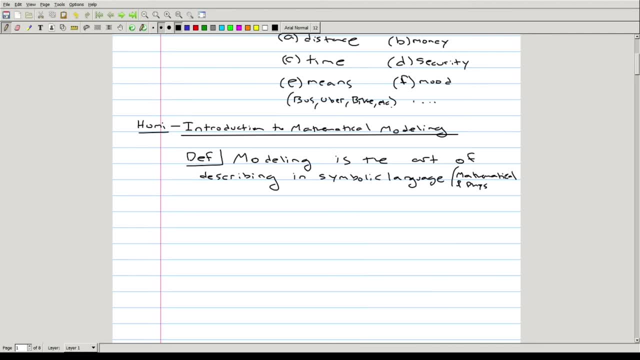 Log Halo, the idea of like we were told one let's drop down Because you're over there. You shouldn't say: over there. You know Zach says: Tell your brother relations, All of you. So you know Hebalance that with people doesn't mean they're assets that you don't team up with a lot. 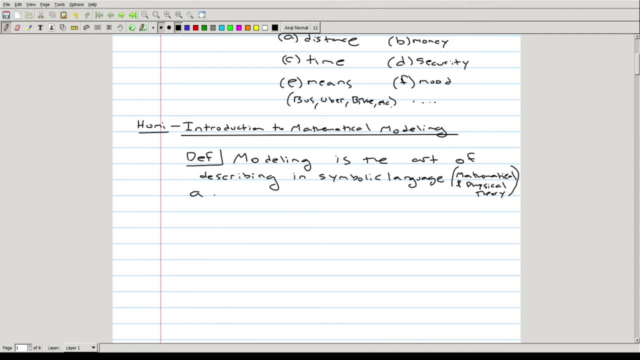 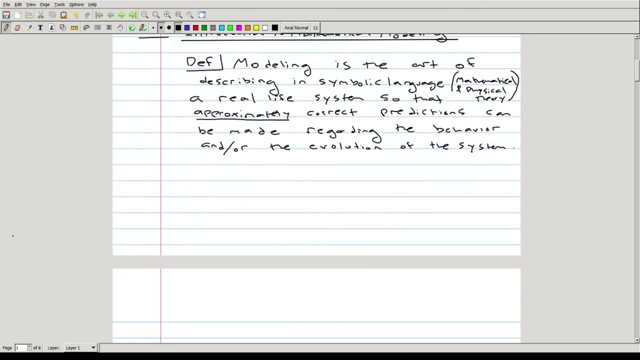 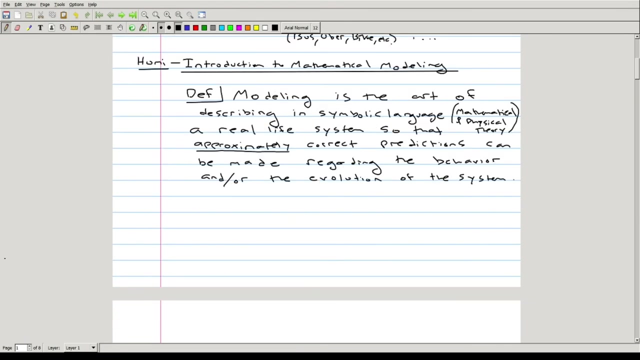 a real-life system so that approximately correct predictions can be made right away regarding the behavior or the evolution of the system. And there are a number of different ways here that we want to make from this definition, The main ones being that modeling is an art. 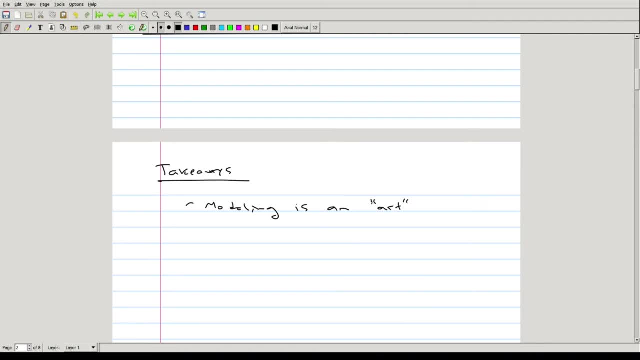 And what that means is that there are no rigid rules Outside of the confines. we can't use any kind of physical theory, Right? So that's all we can do. We don't have to use any kind of independent logic to say that this is our own. 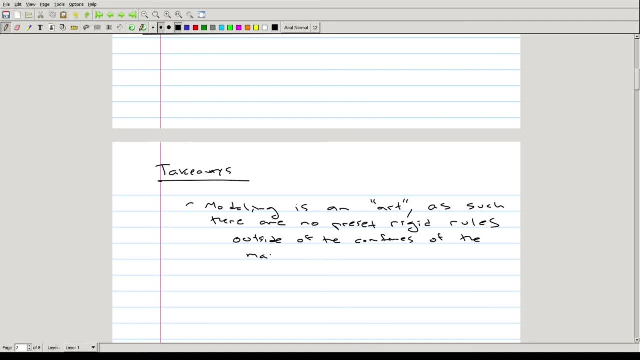 model of the system Right, And that knows that this exists right outside of the confines of the mathematical theory- We could also say physical theory here as well- that you are using and that's the way that this is operating Right. 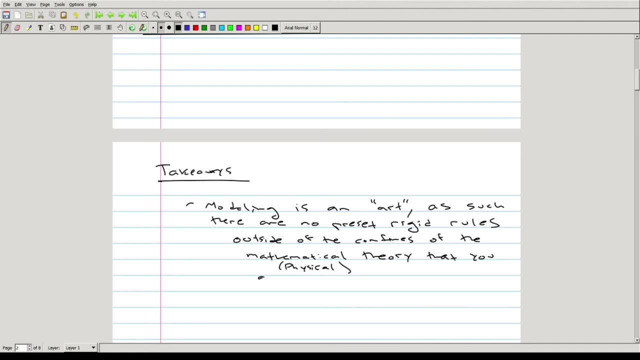 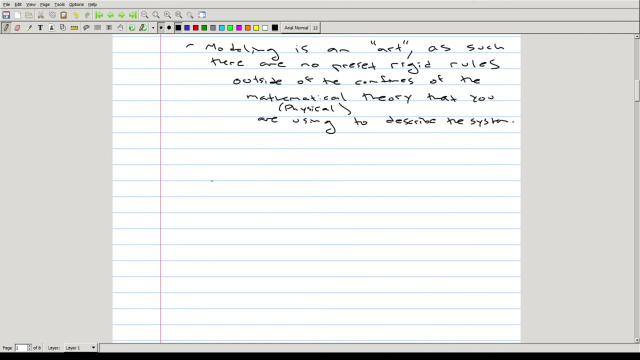 So it's like you're not To describe the system, And this is a very, very important point. It really is an art, and it's an art that you kind of, you develop over time so you become better and better at it over time and with time and practice. 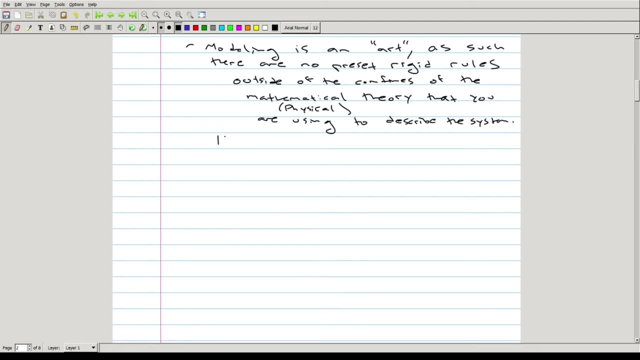 And I also want to point out that, however, here there are patterns. These are patterns of best practice That are common to good mathematical models, or to just good models, And these help avoid many pitfalls that are common to creating a mathematical model. 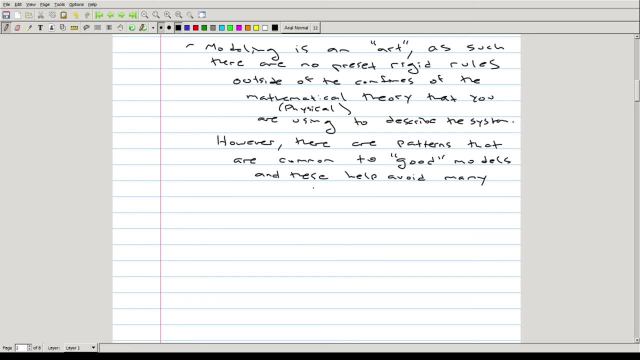 So again, I'm just going to go ahead and start off, So with a simple formula, I would say the following: So let me know if you have any questions or if you just have something that you need And if you can, please let me know. 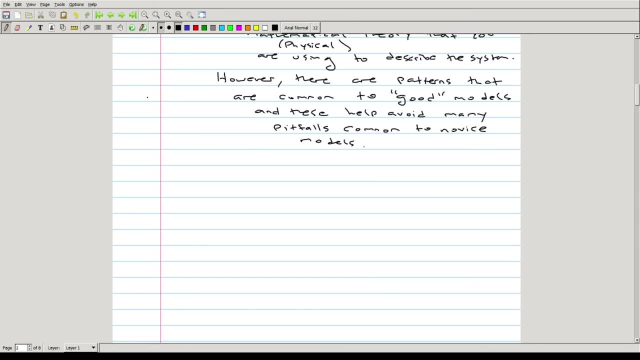 The other takeaway that I want to give you- And then I want to point out a few things. point out about this definition- is that correct predictions usually does not mean 100% accuracy. All mathematical models have limitations and, as such, it's up to us to create the 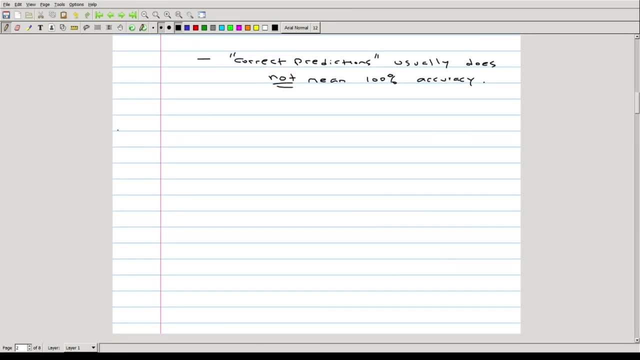 creation of the model. It's up to the creators of the model, those creating the models, to clearly state and investigate these limitations. And I should also put the user here as well, because many times you can use a mathematical model and not be the creator of the mathematical model. 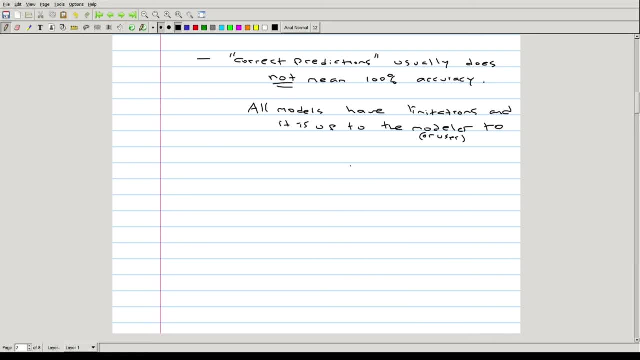 But, regardless if you're using a mathematical model or you create one, you have to determine the limitations and clearly state the limitations. Okay, All right. All right, I think that's it. That's it. The other thing that I want to point out when it comes to this correct prediction is that 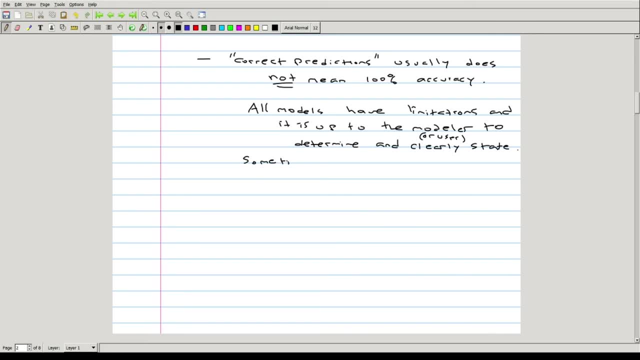 sometimes several models describe the same phenomena. Sorry, I think it's a really good question. What is the correct deadly phenomenon? Let's see, With varying degrees of accuracy, complexity. Sometimes a model that is too complex may be a more accurate description of reality. 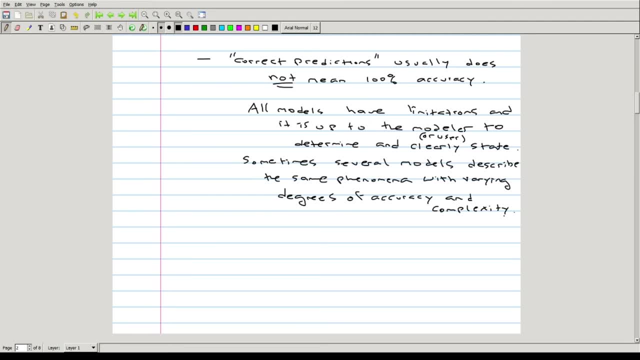 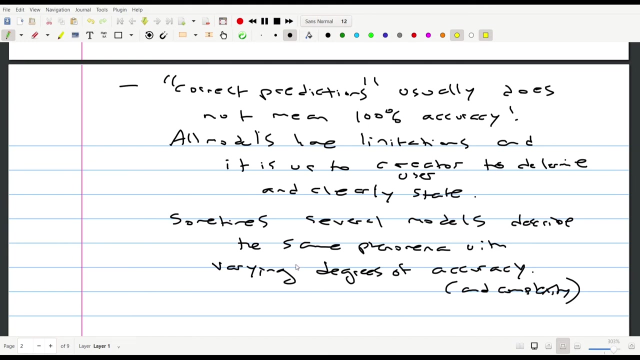 but be very, very hard to apply, and a simpler model will actually describe the real life phenomena in a much more accurate enough way. It'll be good enough, and what I want to do is give you a very, very, very good example of this- And I won't be getting too deep into the mathematics, because the mathematics does go very deep. 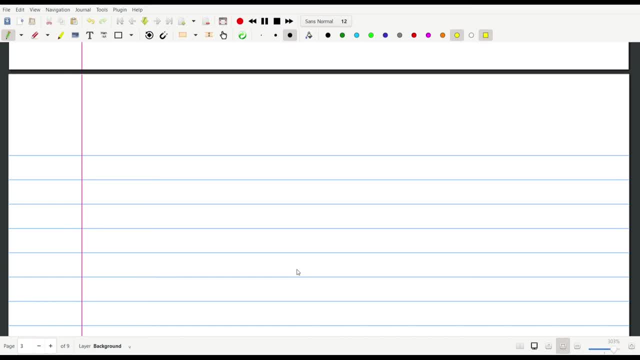 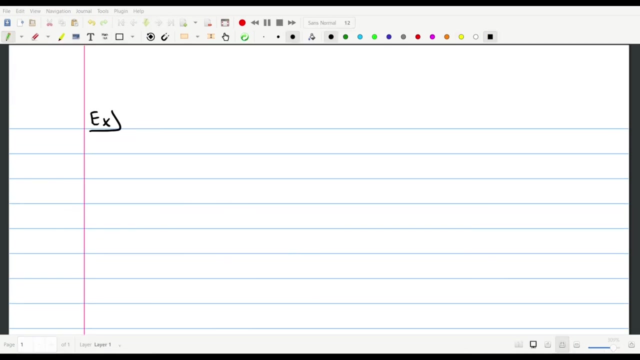 However, what I want to do is just kind of give you an idea of an example of this difference between similar mathematical models describing similar phenomena and how certain phenomena can be complicated in certain situations but be a better model of the real world. And, specifically, what I want to do is look at the example of waves, the wave equation. 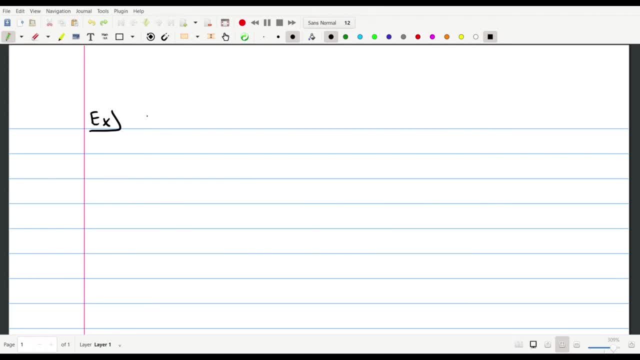 The wave equation takes different forms depending on the application that you're considering. The most basic wave equation, and many times what someone means when they say the wave equation is the linear wave equation. I'm going to call this the basic model and then the more advanced model. 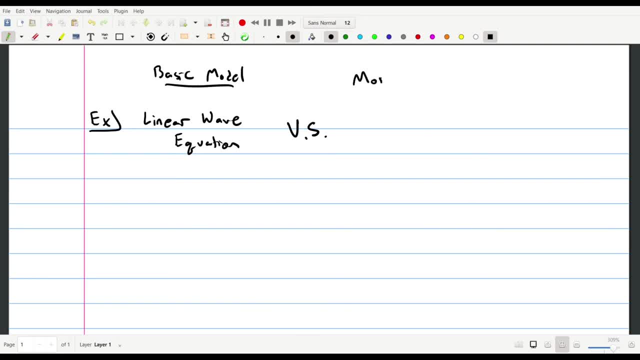 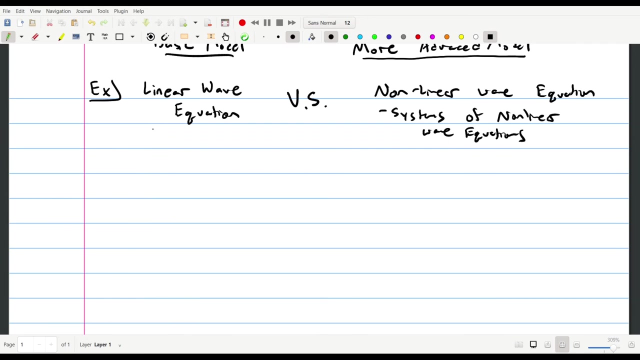 Okay, Okay, Okay. The next model over here will be a non-linear wave equation, Or even systems of non-linear wave equations. Okay, Okay, Okay, Okay, Okay, Bye, bye. so I'll consider the 2d linear wave equation, just to be exact here and this: 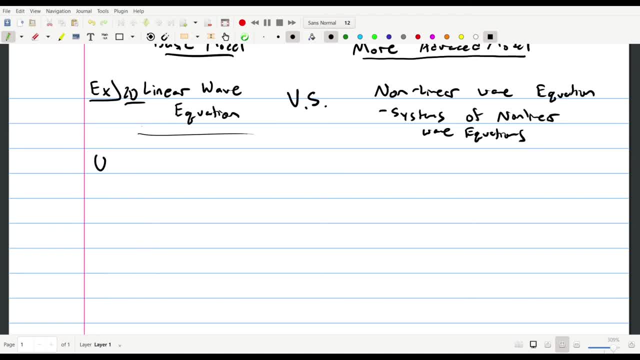 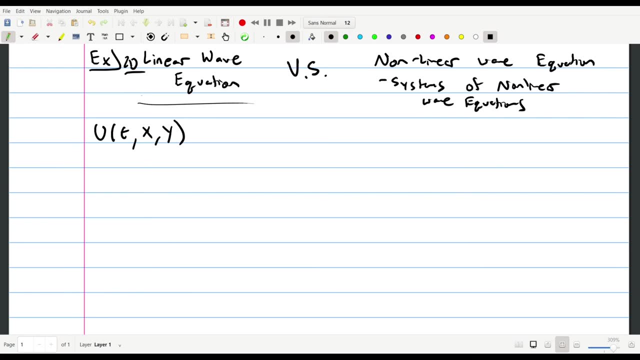 describes, say- I even think of it almost as like a membrane, where the displacement function of the membrane U depends on T, and say on two Cartesian coordinates, x and y. we can show you in some vector calculus that the rate of change of the rate of change of the height of the membrane is the 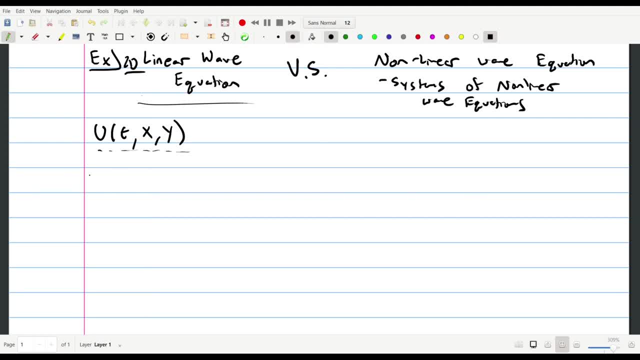 acceleration given xy point on the membrane- this is the second partial derivative of u with respect to time- is directly equal to the wave speed squared times. second partial derivative of u with respect to x, plus the second partial derivative of u with respect to y. this is an equation that you may have briefly seen in a multivariable count. 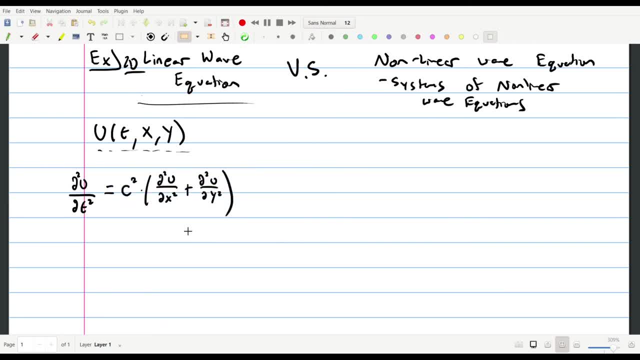 course you're definitely not expected to know it, but hopefully you have reviewed your partial derivatives and essentially what this is saying is an expression of Newton's law, Newton's second law of motion for every given point on the elastic membrane. so really, if we draw a coordinate system, 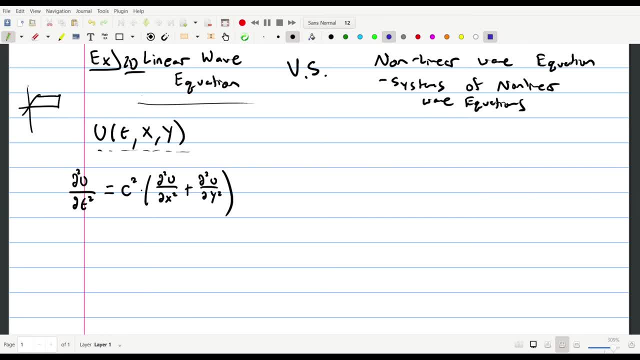 we think of our membrane as, say, being some surface that goes up and down in various points on the surface. what we're studying when we solve this is exactly the behavior of linear waves. now for large deformations in the membrane. this is not the correct equation to use to 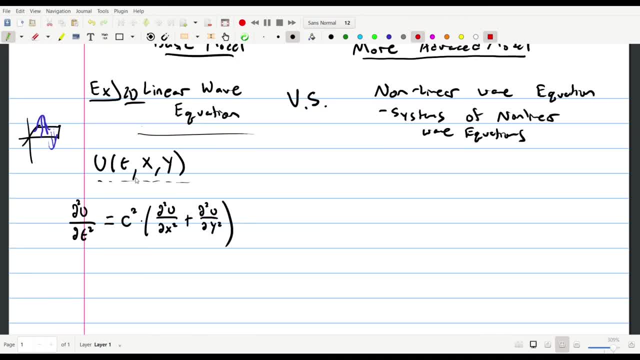 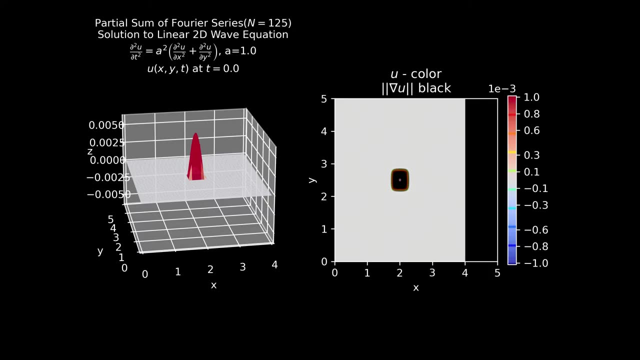 model propagation of waves. but for small deformations, this linear wave equation turns out to be a very good model of propagating waves. what I want to do is show you this for a given initial condition. so what you see plotted here is a display of a given 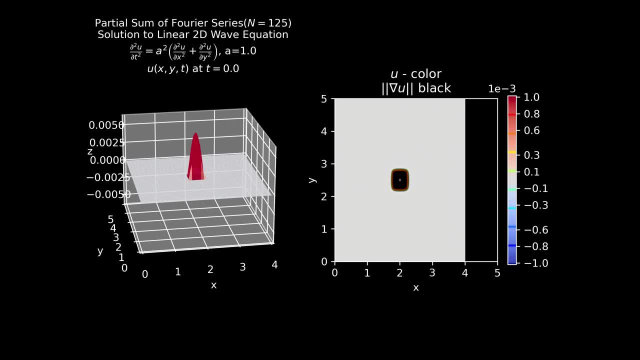 initial condition and the left is the graph of this membrane- initial condition that we're putting on the membrane, and the right is a contour plot showing both the displacement of points in the membrane in color, so red and blue, and the gradient in black, so the magnitude of the gradient. 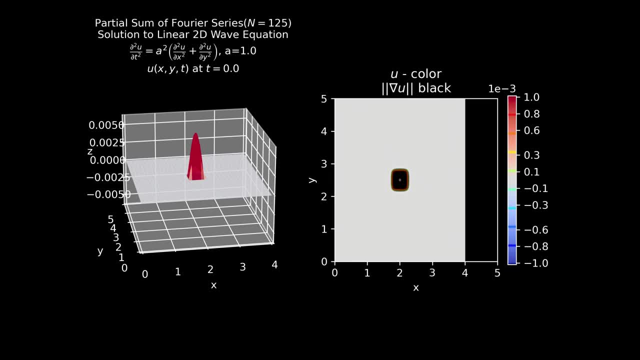 of this displacement, and I'm going to plot the exact solution of this equation as it depends on time, for t from 0 to 20, and so we can see that the wave proceeds, bouncing off the boundaries, and we're getting a very good picture here of exactly what the solution to this 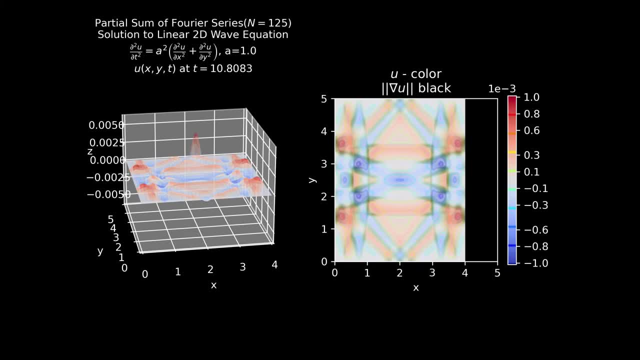 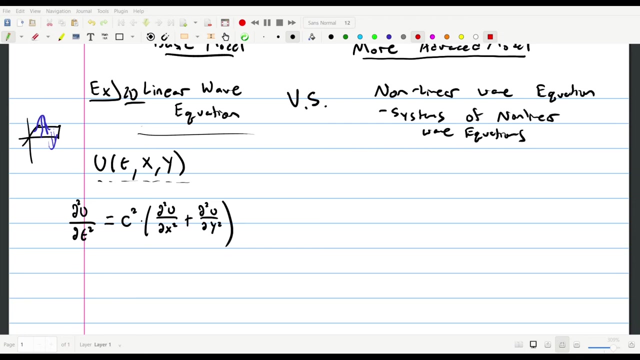 distribution looks like. so, believe it or not, this is actually one of the more basic models, even though solving it actually requires a substantial amount of mathematics. the linear wave equation is not not typically the best model to use, and there are actually many more advanced nonlinear wave equations that 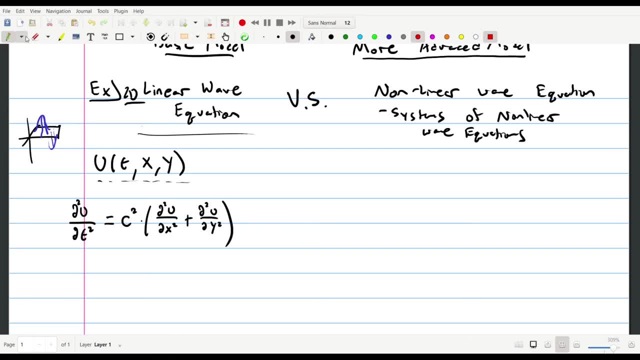 are actually better suited to model reality. I'm not going to write the equations down right now, but I will name them. one of the main ones is the Corwig-DeVries equation, which shows up in many areas of modeling advanced fluid flow as well as. 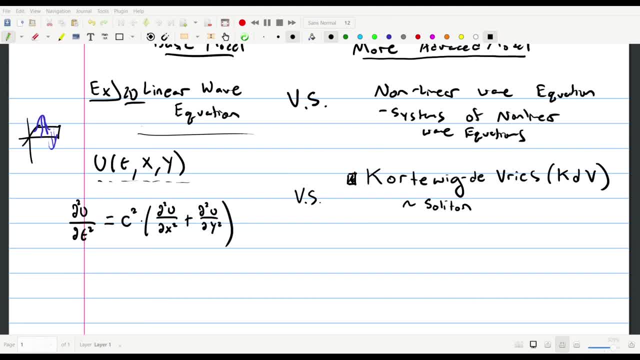 in many areas of quantum mechanics. these are sometimes called KdV type equations of KdV equation and, believe it or not, we'll be able to use some of the methods that we're going to develop in this course by the end of it to actually solve this equation and equations like this. 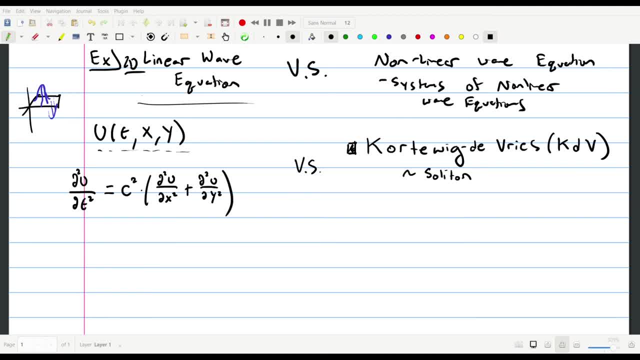 so this is a very, very important system of nonlinear partial differential equations. another very, very, very important system of non-linear partial differential equations are the so-called Euler equations of gas dynamics. These are extremely important in studying and understanding the behavior of shock waves. and before we get into the procedure of dealing with these methods, 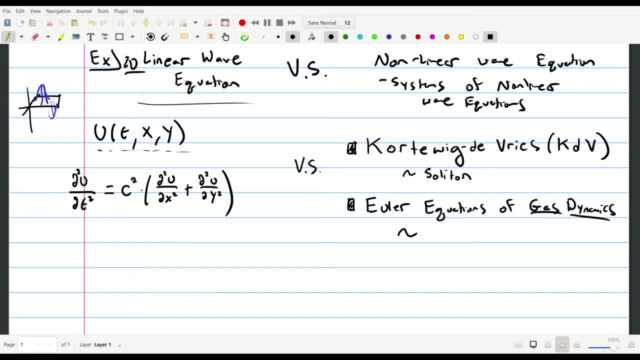 shockwaves in gas flow over various different geometrical objects. These equations are much, much more complicated than the standard linear wave equation, and solving them exactly analytically in three dimensions is still an open problem in mathematics. However, there are ways of numerically solving both these types of equations. 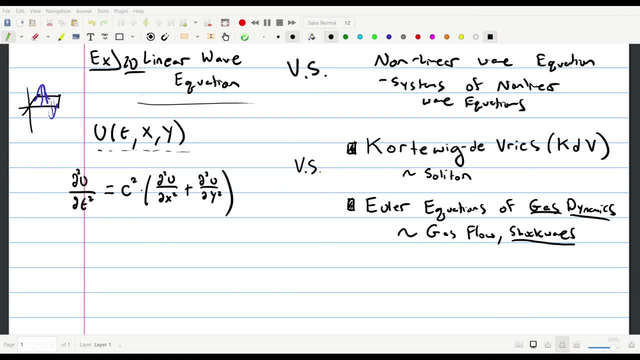 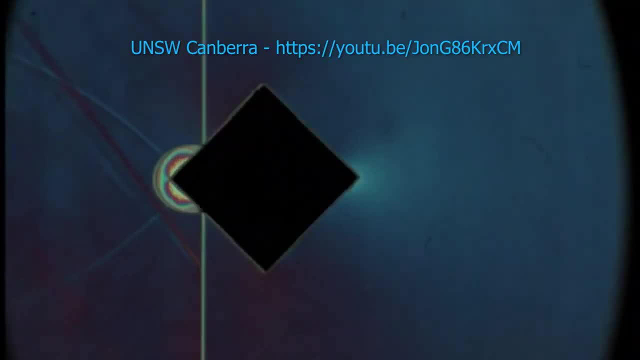 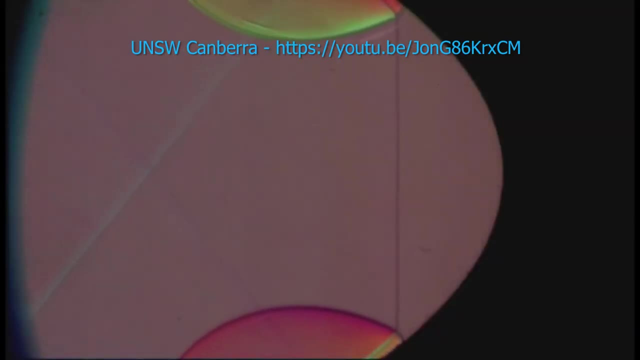 specifically the Euler equations. What I'm going to show right now is some experimental results and then corresponding numerical solutions of the Euler equations for different scenarios. So what you see right here is experimental results from the University of New South Wales showing a shock wave proceeding through. 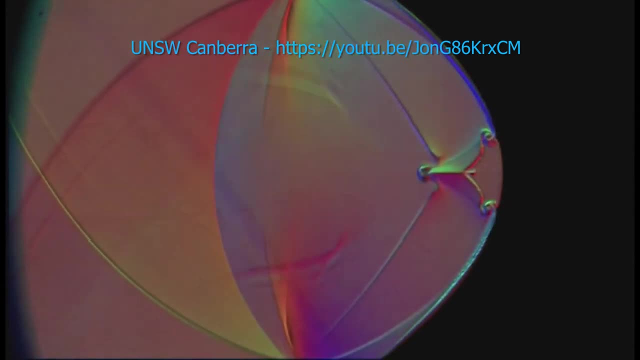 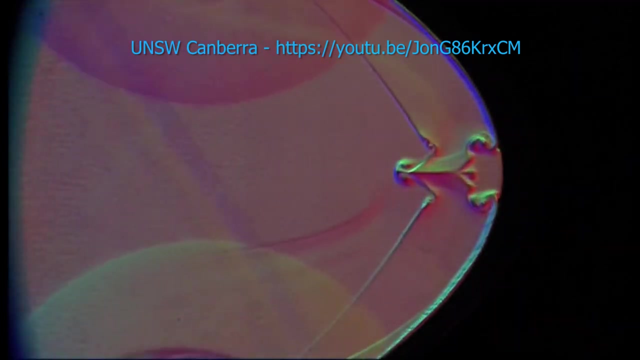 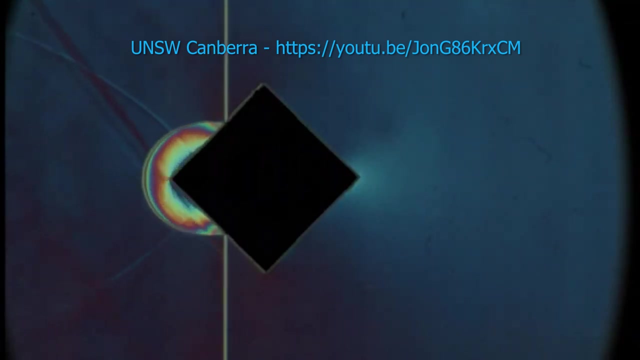 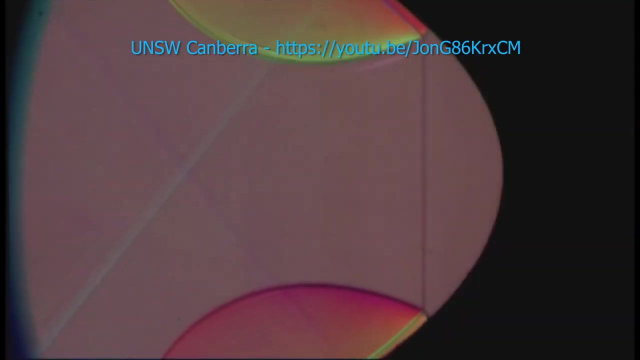 the material and then interacting with the boundary, and you see two separate videos here. The first video is a shock wave interacting with a square obstacle and the second video is shock wave proceeding interacting with a parabolic boundary. Both videos consider very complicated behavior of the shock wave. specifically, 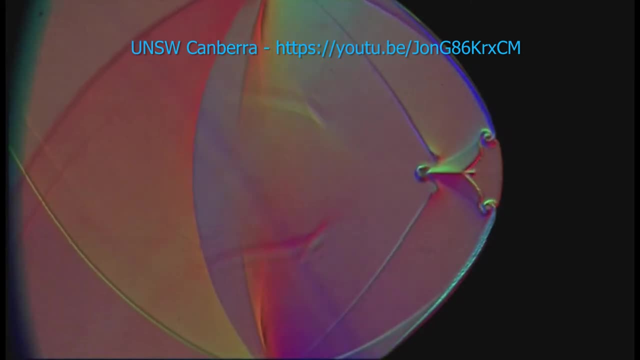 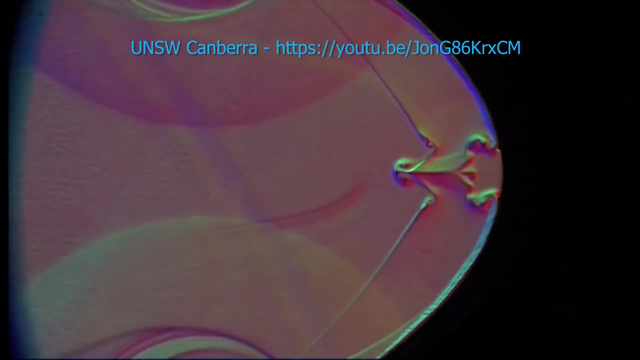 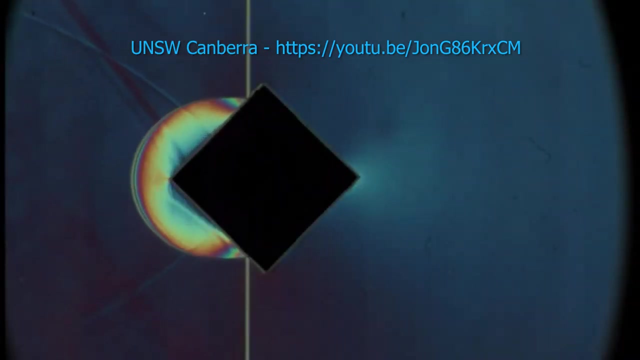 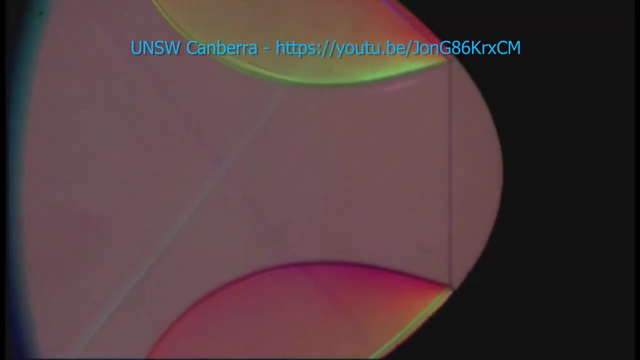 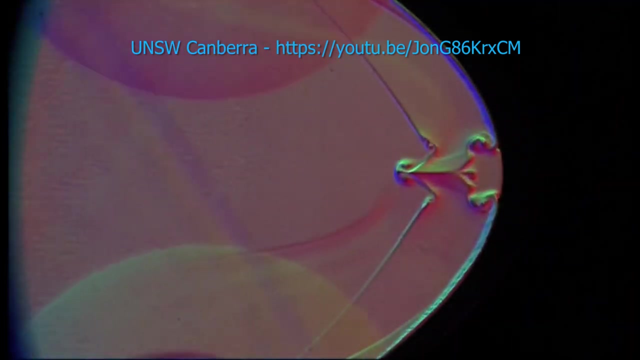 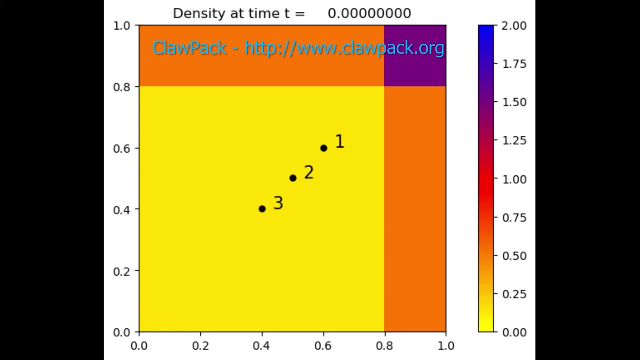 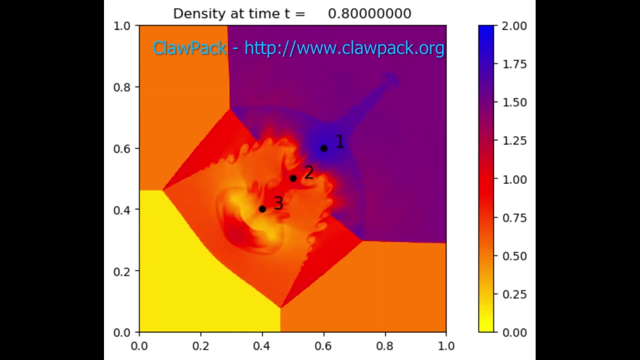 the formation of eddies or rotational flow in gas. This is behavior that can't be adequately modeled using a linear wave equation. However, the system of Euler equations can very accurately reproduce these effects very, very nicely, And what you see here is numerical simulation of the solution to the Euler 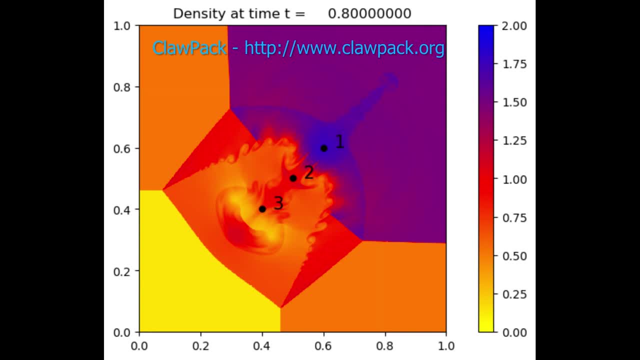 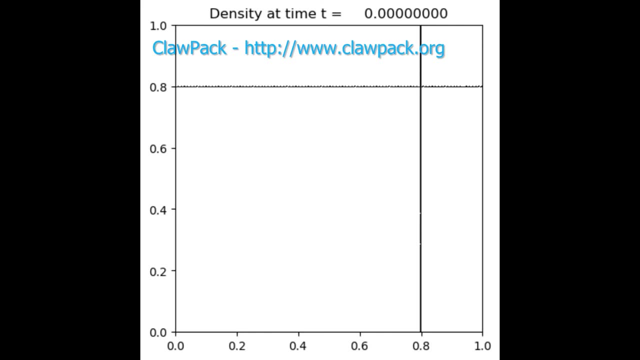 equations, which is recapturing all of this very complicated behavior that we're seeing in real world experiments. But this is coming directly from a computational simulation of the Euler equations and we're going to go through our analysis and then go on to solve this problem. 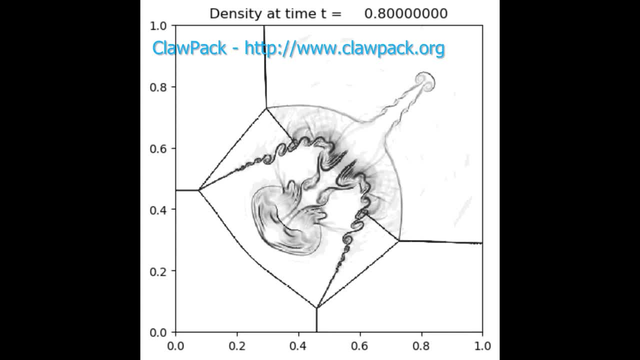 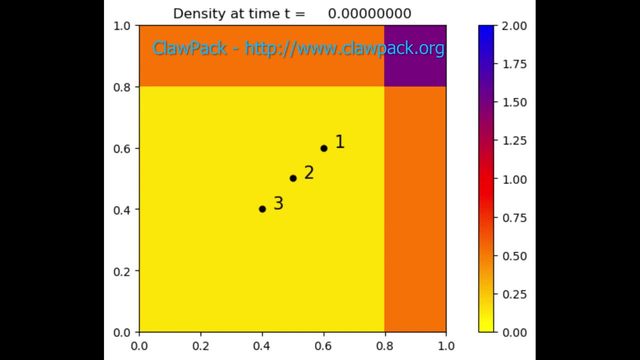 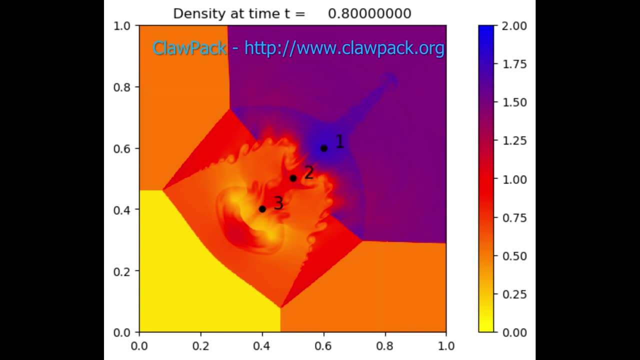 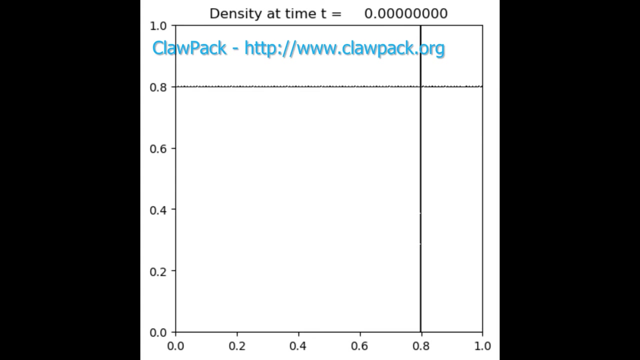 the correct mathematical equations of gas dynamics, um, and i think it's very, very, very convincing uh, and you know you're seeing formation of these eddies, uh, as well as uh all of the real world results in terms of, uh, how the shocks actually do uh propagate through the material uh the gas. 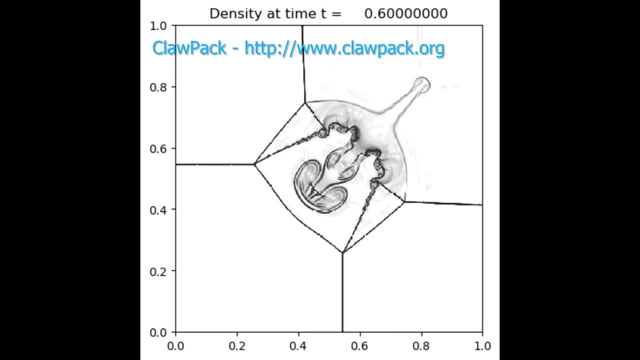 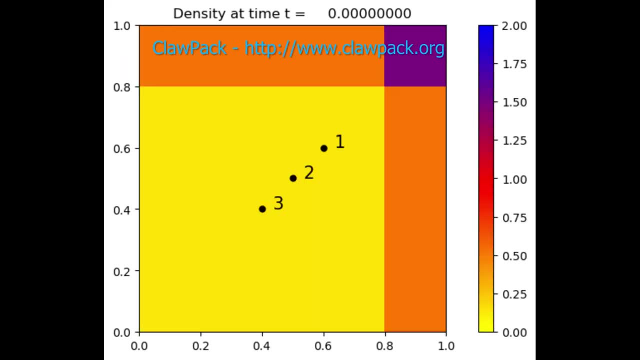 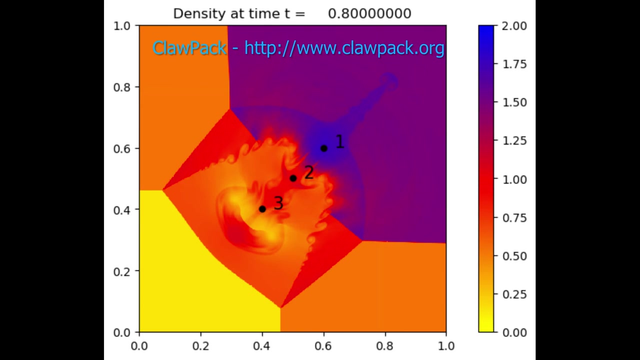 uh, in the real world, uh, experimental results. so i think this is very convincing, very shows a very, very strong evidence right that sometimes using the more advanced model, even though it's more difficult to get computational or analytic results, is very fruitful and very, very important to consider. 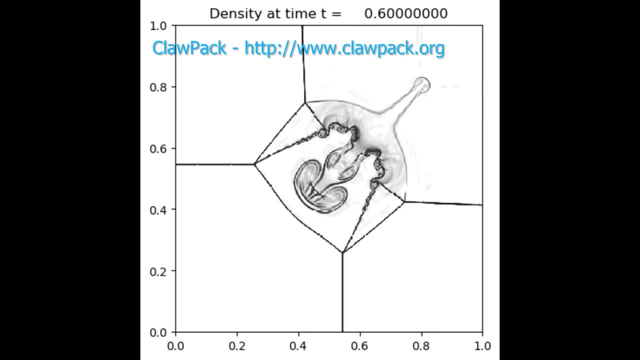 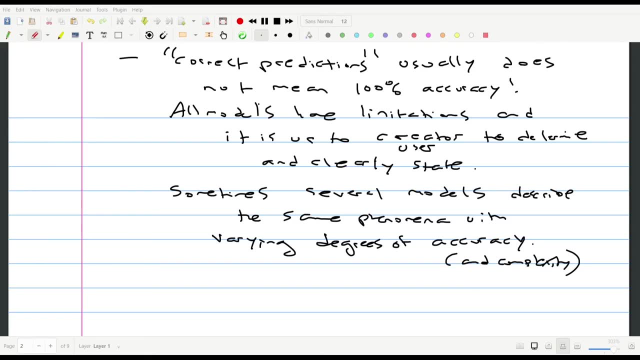 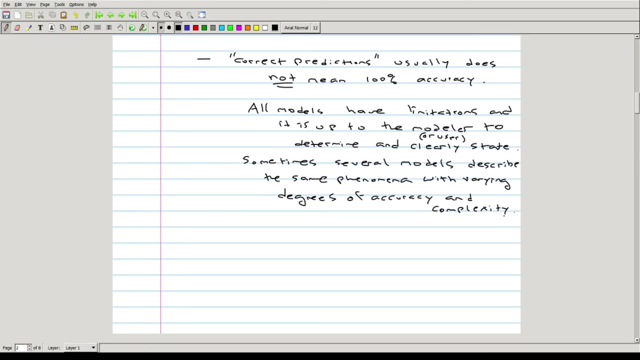 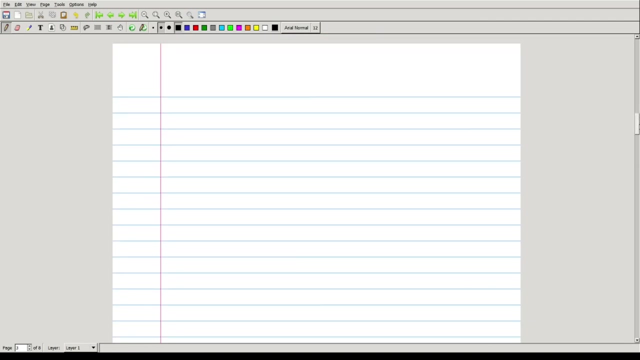 so i have one more example that i want to give of this uh uh idea of, you know, relatively basic model compared to more advanced model. this is the example of gravitation theory, this the theory of gravity, and there are two main theories of gravity. there are many theories of gravity that have been developed. 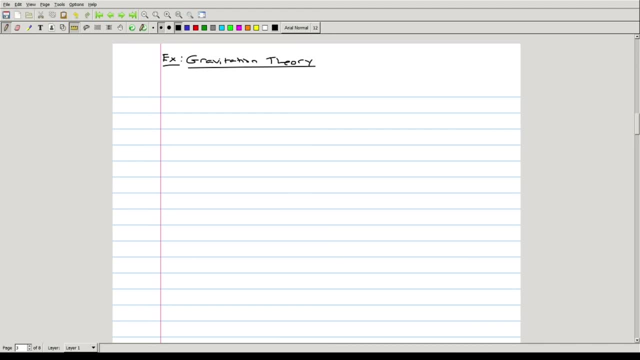 but the two main theories of gravity that have been uh developed by by physical scientists and by humanity are the newtonian theory of gravity, or newton's theory of gravity, and that of uh einstein's theory of general relativity. albert einstein, you. 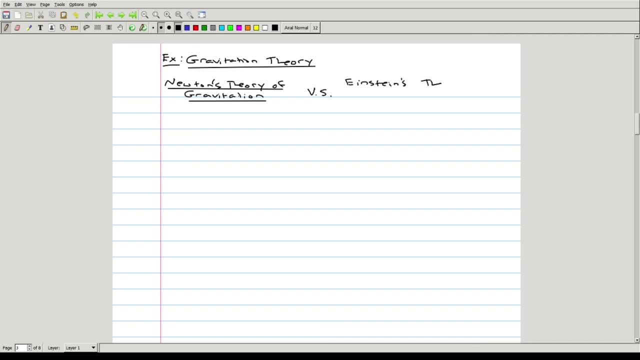 you, you, you, you, you you. And I'll also include- because I glued some of these together- some special relativity over here. I'll include Newton's theory of mechanics and gravitation. So we'll start out by comparing and contrasting these two major developments in scientific. 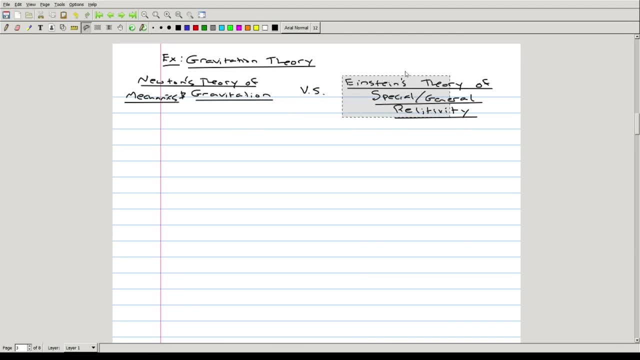 understanding of mechanics and gravitation. Okay, Newton developed his theory around 1687, and there is some controversy between whether he discovered parts of the theory and others discovered parts of the theory, like Robert Hooke. But we'll avoid that controversy for now by just saying it's Newton's theory of gravity. 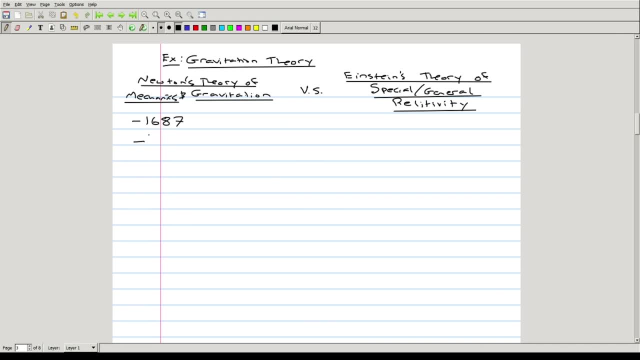 and start out by saying this is an extremely successful theory of mechanics and gravitation. It was so successful, in fact, that this theory was actually used to achieve the Moon landing. Okay So, Okay, So, Okay, So, to expedit that. 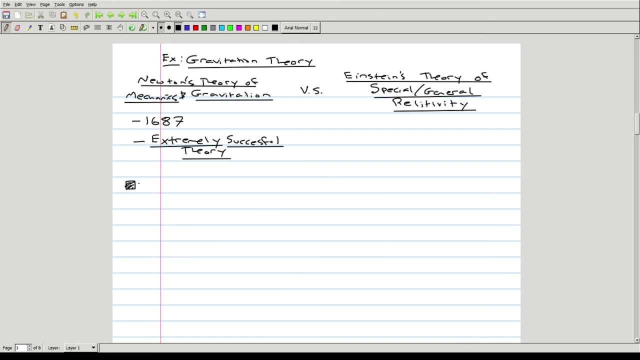 So it's really a long story again. Okay, because of connection issues, you can see the удивinableness being characterized in Gemini, which I'm sure everyone knows as the Lunarius. Okay, It's also used by current day astronomers and astronauts in current day missions, where 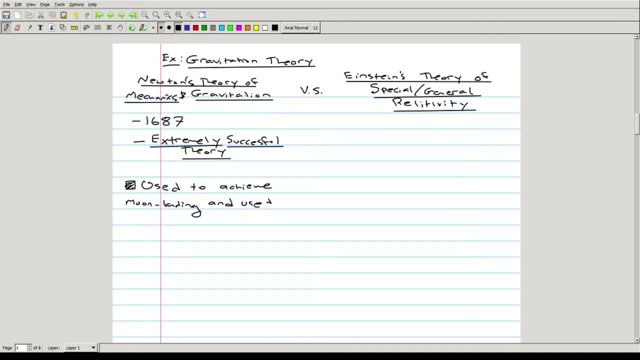 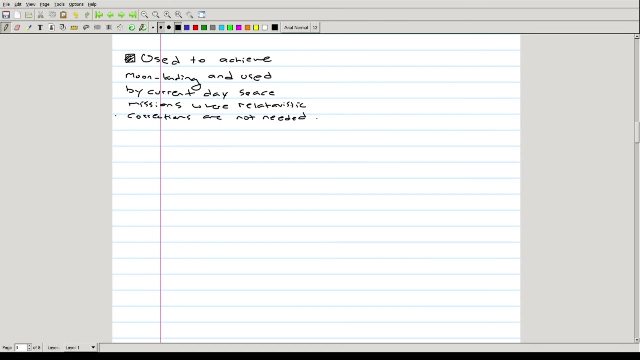 relativistic corrections are not needed. We can use Newton's theory of gravitation to actually prove, mathematically prove, Kepler's three laws, And this is something I do in my graduate engineering mathematics class. So Kepler's laws, you'll remember, are three main laws of motion, one being the planetary orbits. 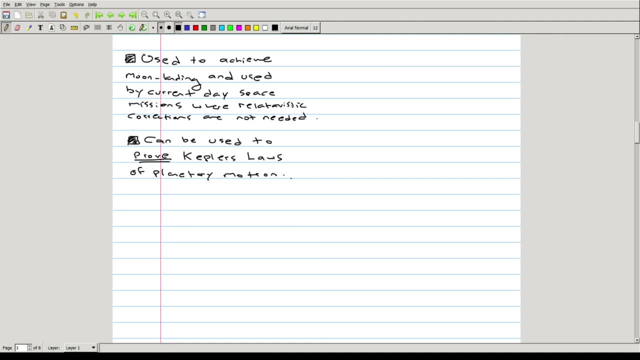 one being the planetary orbits and the other being the planetary orbits. They follow what are called conic sections or ellipses, parabolas or hyperbolas. They also relate the area of traversal to the period of motion and give you a relationship. 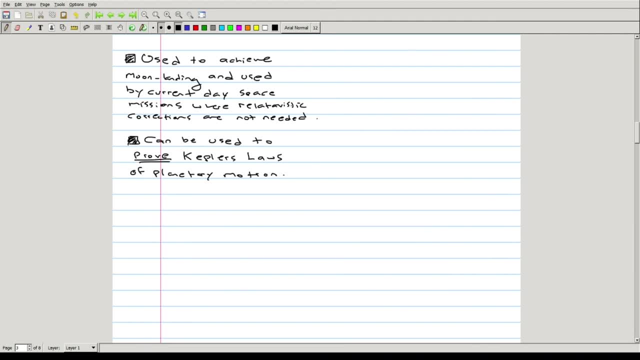 between the period and the length of the semi-major axis of an orbit of a planet around a massive body. This theory is also easier to apply and use than relativity. I put this in quotation marks here because there are some caveats, but in general it's much easier to apply. 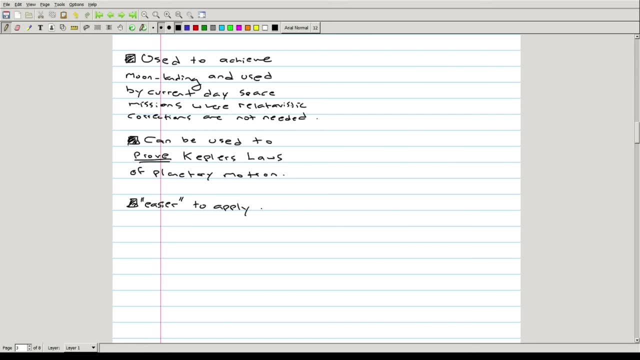 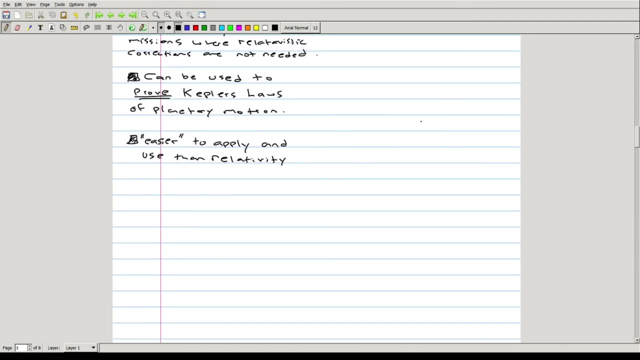 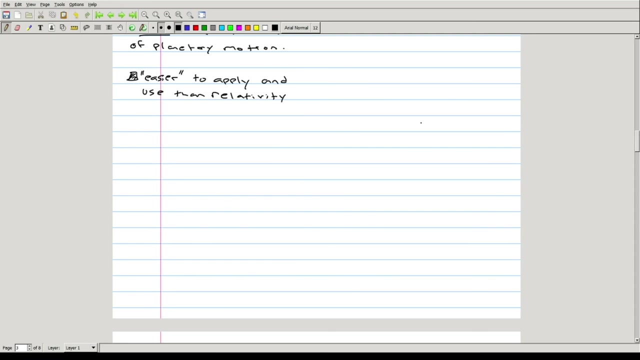 and use than relativity. There's бан: einste glßt, einste sch a herr. But in Einstein's theory of relativity, However, there are, for all of the benefits of this theory, there are some major limitations. Of course, there are things you could do. The Economics of Fisher's- The whole topic of science used to support grammar rules as well. you can try to run some exams and get some information And tool for attendance Ep unmissed. Isn't a worry for задv. Surely keep it up to date. 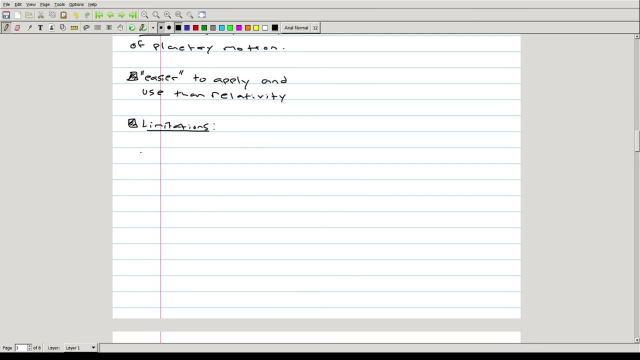 ab selv cs. The most historic and biggest limitation was its failure to calculate the precession of various planets, of the perihelion of various planets. Specifically, Mercury's prediction is way off. Thank you for watching. Thank you for watching. Thank you for watching. 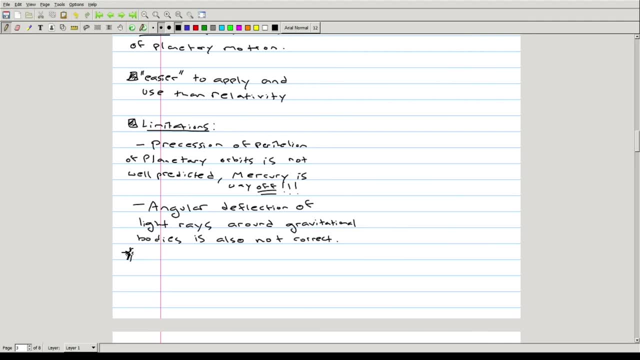 For instance, if you have the sun here and you're on the Earth right here, light rays as they pass the sun, if they're coming in like this, end up getting deflected by the gravitation of the body. So, for instance, if you're looking at a star and you see a star in this direction from the Earth, 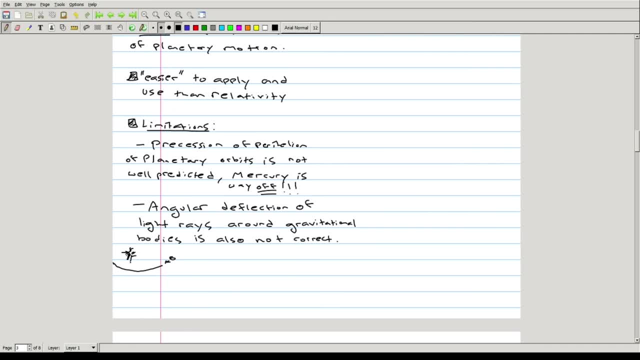 the actual location of that star is over here, And this is because of the gravitation of the sun. It actually deflects light rays. This is not well predicted at all by Newton's theory of gravity And in general for Newton's theory of gravitation. errors build up over time. 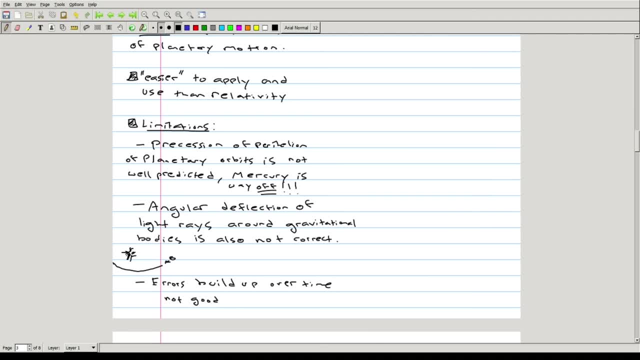 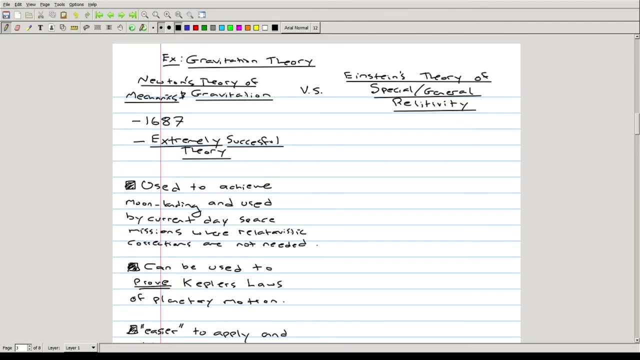 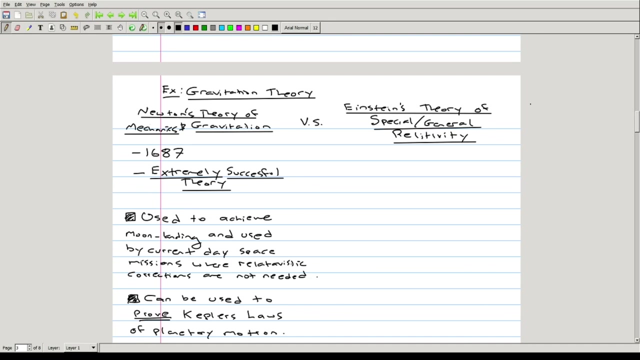 Which means it's not good. And you can go back to law of gravity to say that gravityDon Winter has refuted for long timesp Ve or for predicting over long time spans. This is a summary of Newton's theory of mechanics and gravitation. 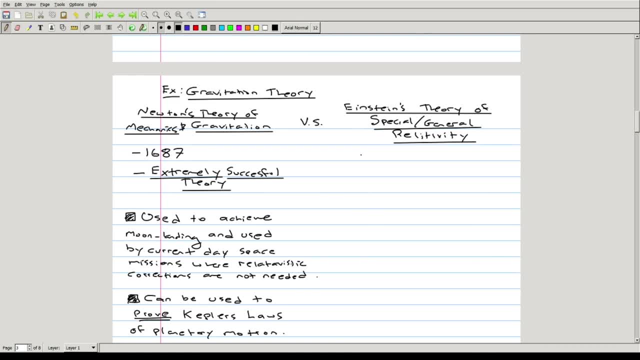 This is the summary of Newton's theory of mechanics and gravitation. that can introduce new theories and new assumptions. on it other hand, we have Einstein's theory of special and general relativity. Einstein published his papers around 1916 and this is also an extremely successful theory of. 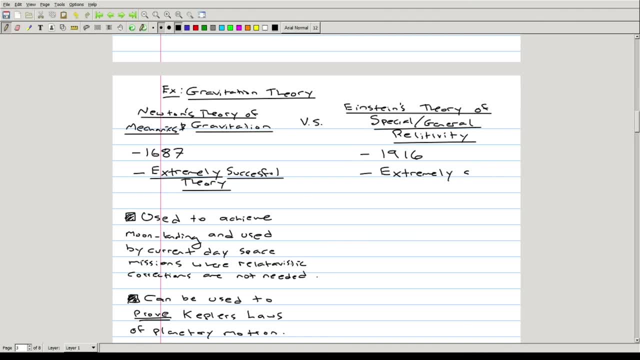 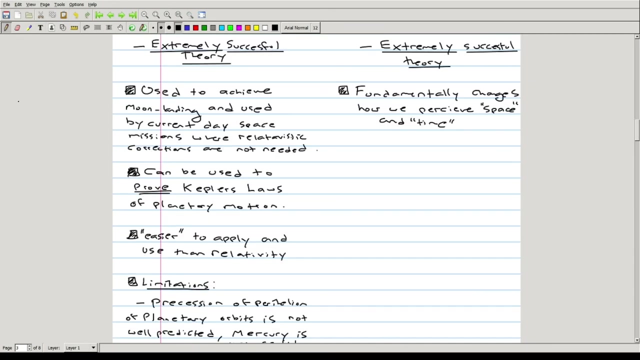 gravitation. This is definitely a very, very, very big theory because it fundamentally changes the idea of space and time. Einstein's theory of general relativity is actually required to create modern GPS systems and a number of other modern systems. Einstein's theory of general relativity is actually required to create modern GPS systems and a number of other modern systems. 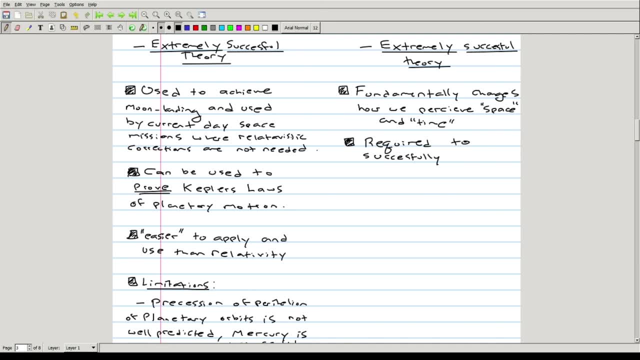 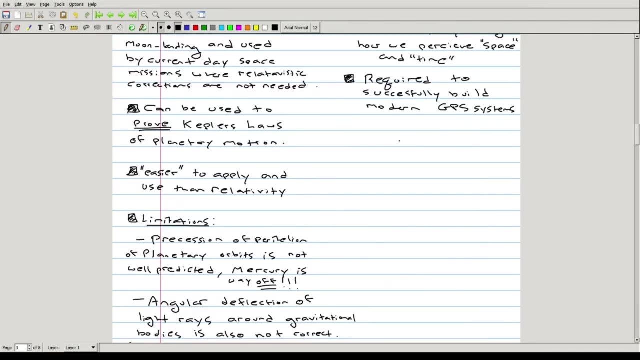 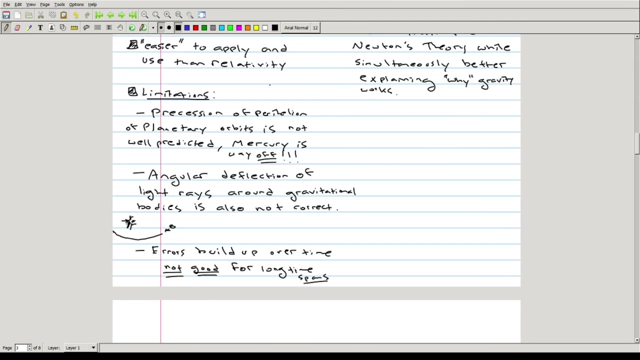 you and in general. uh, by greatly overhauling a lot of the fundamental ideas of space and time and fundamental ideas in physics, the theory addresses and explains and corrects the limitations of Newton's theory, While simultaneously better explaining why gravity works And in general. 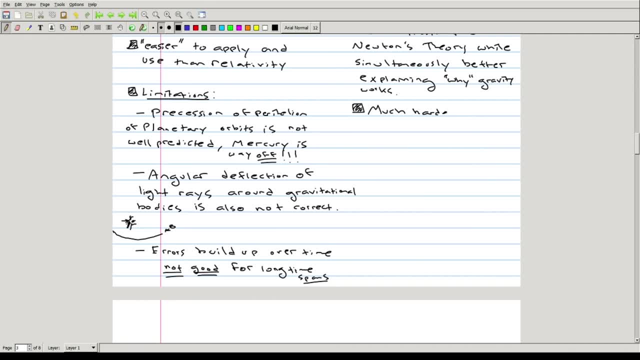 it's much harder to correctly understand the theory of relativity, Apply and solve problems in general relativity. There are definitely some other limitations to this theory as well: Extreme scenarios such as very, very large mass like black holes, and so on. 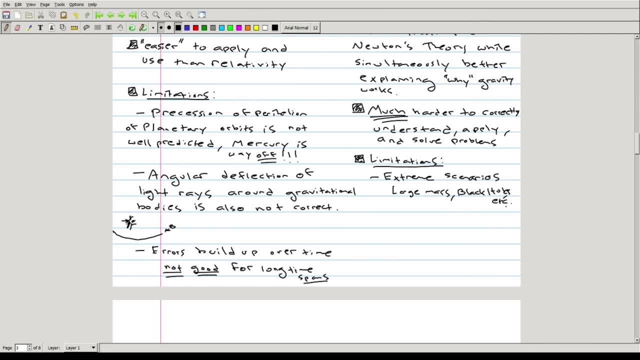 We have complications because there's a fundamental misunderstanding of how general relativity, which works at large, large scales for very large distances and large scales between planets, interacts well with quantum mechanics, which is the theory of the very small, extremely small fundamental particles. 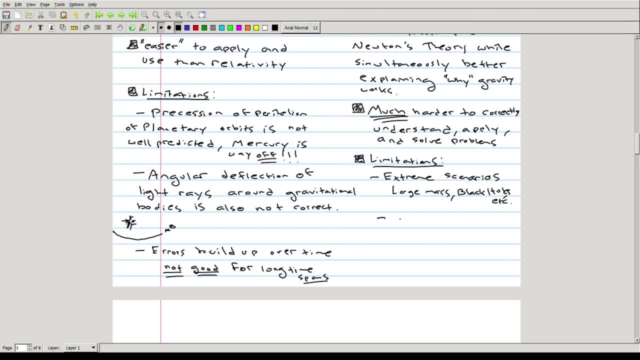 So in general, Einstein's theory of relativity doesn't mesh well with quantum mechanics. This is actually one of the biggest problems in physics right now is to find a new, more physical theory that gives us Einstein's theory of general relativity but meshes that with quantum mechanics. 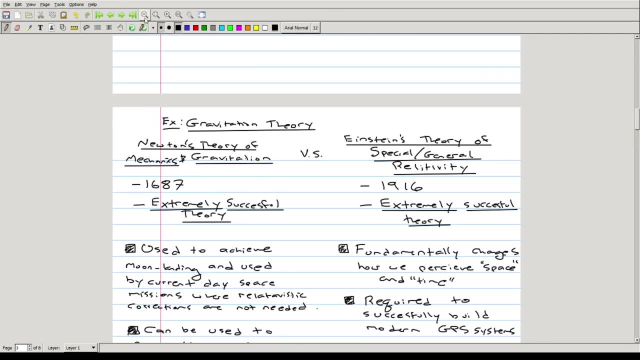 But in terms of just theories of gravitation, the more modern theory- and some people will say the better theory- is Einstein's theory of the special and general relativity. But I wouldn't say that it's better, I just think that it's more modern and it's more accurate. 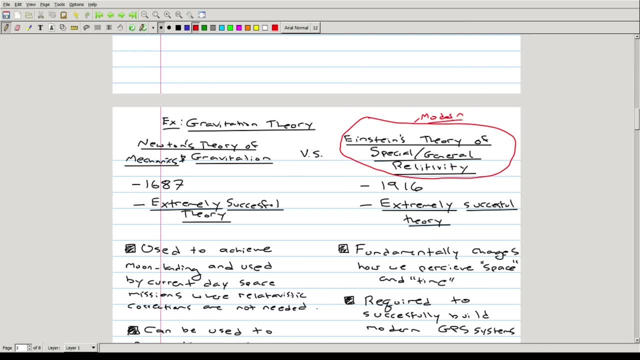 It's a more accurate theory in significant accomplishments- The world changing accomplishments in mankind- have been achieved by both theories. World changing accomplishments have been attained using both these theories. What's also important to note- this is the final note that I'll make on this example- 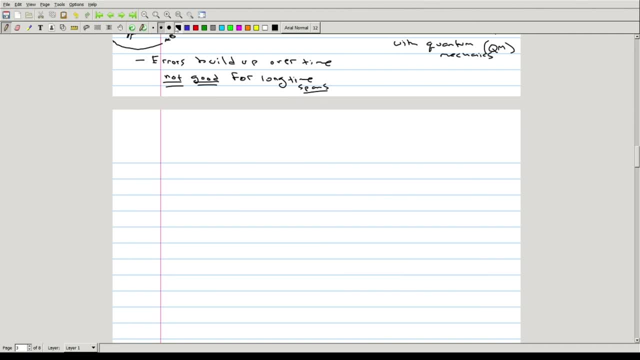 is that sometimes, if you have one theory that's less accurate, one theory that's more accurate, you can address and use the less accurate theory while introducing corrections from the more accurate theory. So for this example, Newton's law, I should say Newton's theory of gravitation. 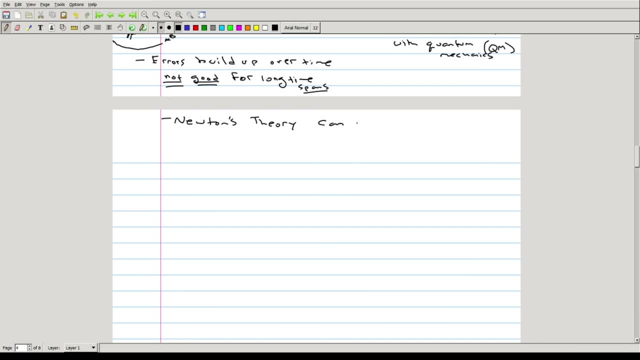 can often be used with, and is often used with, what are called relativistic corrections, Tacked on or attached, Which will correct or correct Newton's laws and add in the corrections that we know are actually true and observed in real life, that can be explained via relativity. 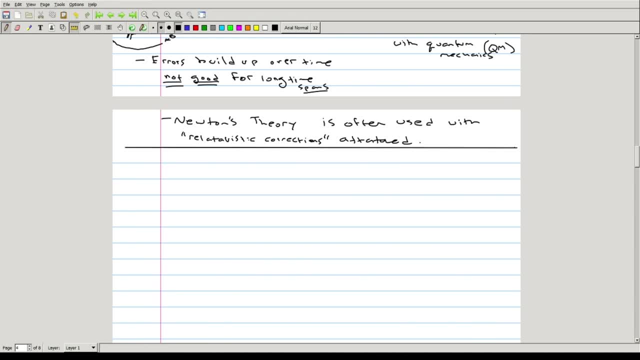 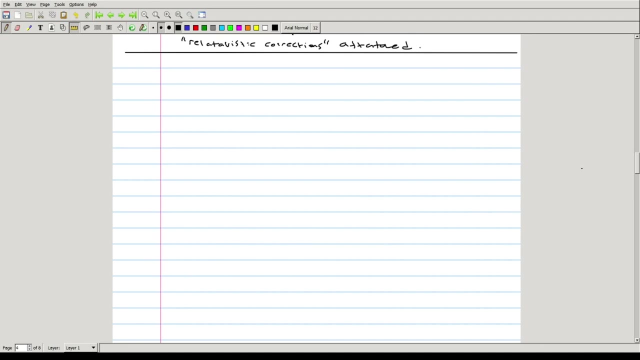 And we'll investigate this a little bit later on in the course, when we get some development into our toolbox, our technique. But the main thing you want to be thinking about thinking of in this course and in general in your learning mathematics, is: 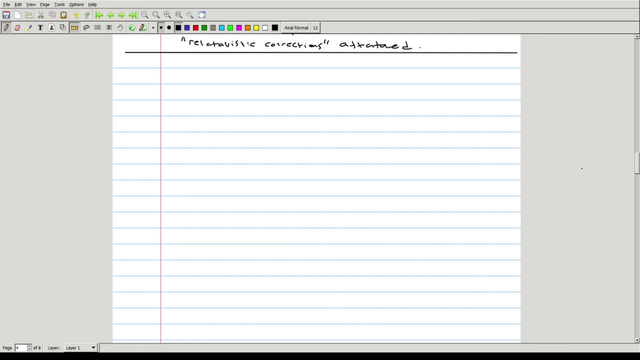 how it's adding to your toolbox for mathematical modeling and for figuring out problems using mathematics. So what I want to do now is just give a quick overview of the general modeling framework and mathematical modeling. You know problem consists of and how it's typically a very large process. 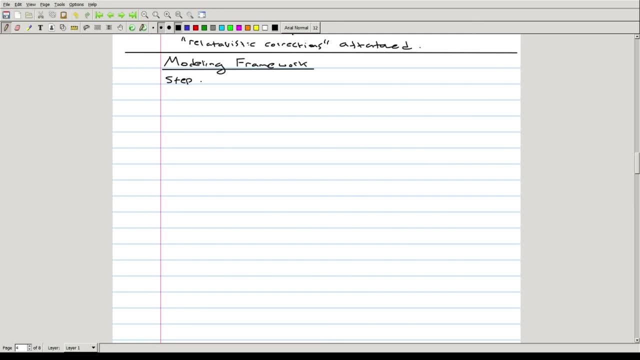 And, just like the previous definition, this process can be found in Meyer-Humey's book and I very strongly recommend taking a look at the book, because it's a very, very nice and extremely detailed and informative summary of how to make a mathematical model, and very, very in-depth as well. 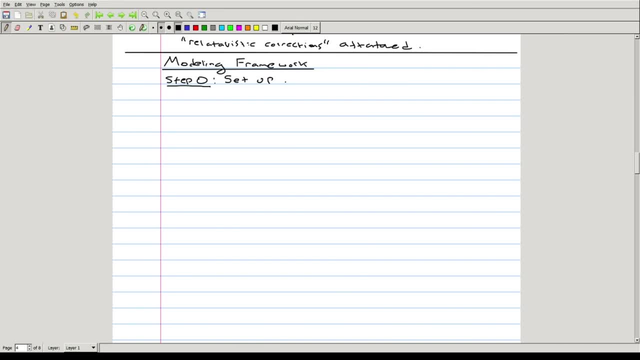 The step zero in this process is to set up as precisely as possible the reasons for constructing the model and its objectives. So, for example, if you're making a model of the weather and you want to predict the weather, do you want to predict the weather for a day? 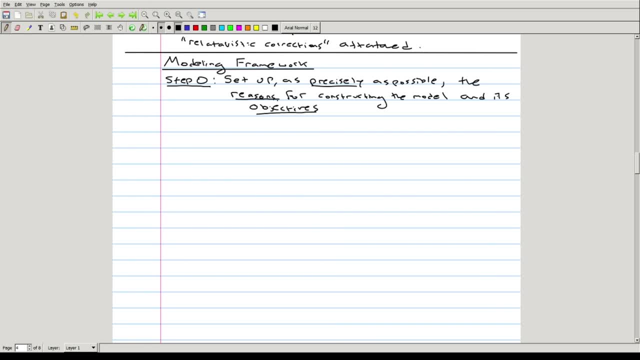 Do you want to predict the weather for an hour? Do you want to predict the weather for a week? Each one of those questions is a different question. They all are very difficult questions, but they all are very difficult questions, but they have very different difficulties associated with them. 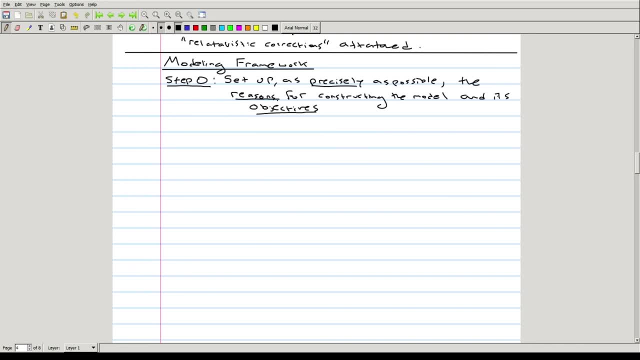 And, as you can see, if you look at your local weather forecast, you don't really get much accuracy, even within a few days, for a weather forecast. So the next step, step one, is to study the problem as it is in real life. 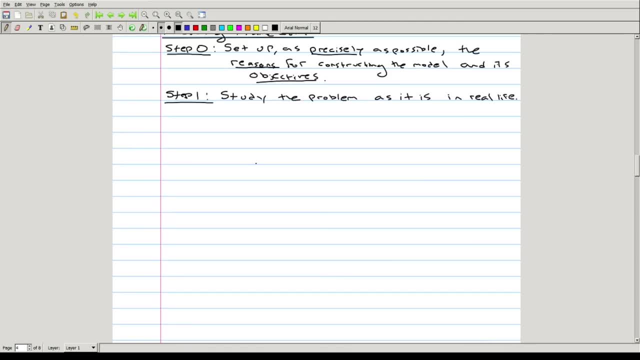 And this involves doing a lot of research to figure out exactly what the problem is. you're dealing with and you know what exactly is going on. It's also setting up for the next step, step two, which is data collection. 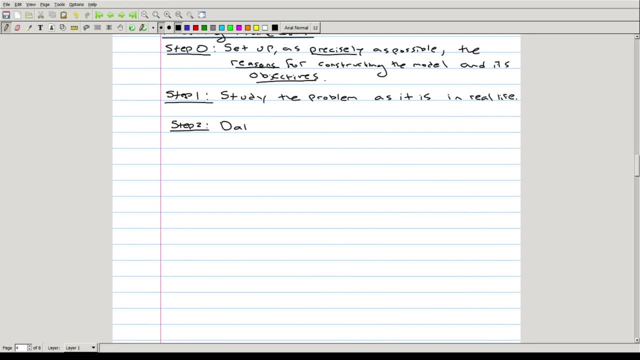 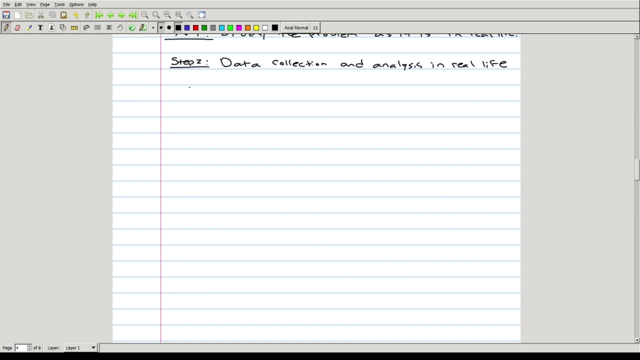 and analysis in real life, And this is where you go out into the field or you collect data from laboratories and you collect real-world data to analyze, And this actually then leads into step three, Where you design controlled laboratory studies. 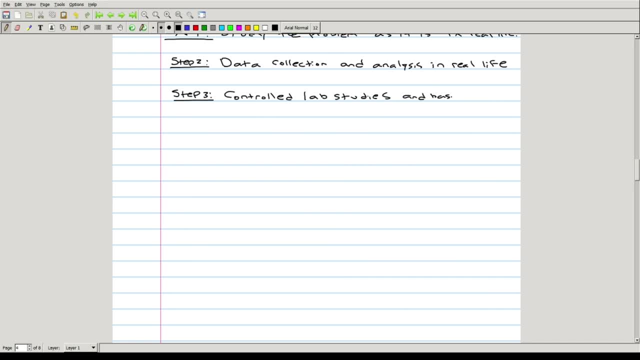 And simulations. And then the last two steps here are step four and step five. Step four is the construction of a conceptual qualitative model, So it will be a lot more complex. So in this example, let's do the final 5 step. 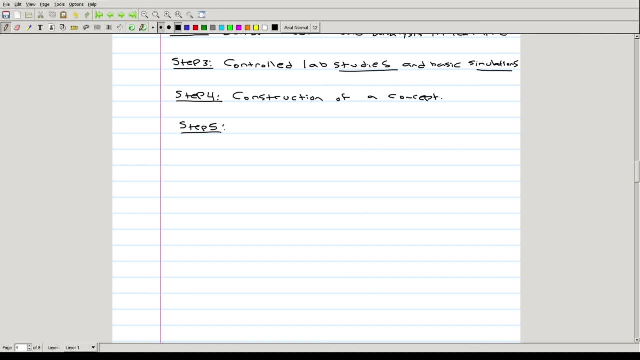 It's not going to be a very detailed analysis of all of it. I'll just do a little bit of a broad analysis And I'll just take a few minutes to have those two steps as a work. So let's say: 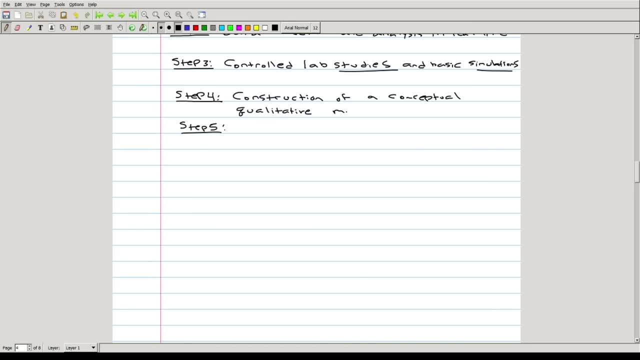 one of the things I like about quantum mechanics in this model is that it allows you to weigh, see the answers of these questions, And you can look at them in this model And notice that I'm using the word qualitative here, not quantitative. 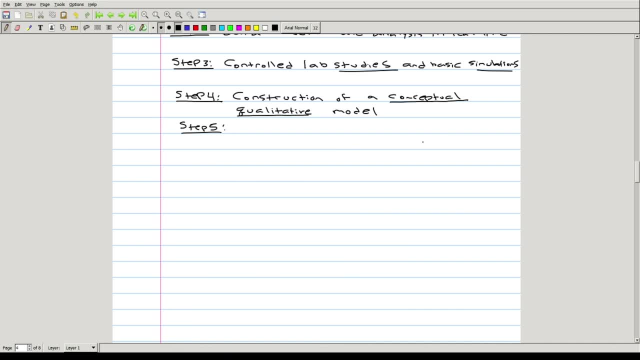 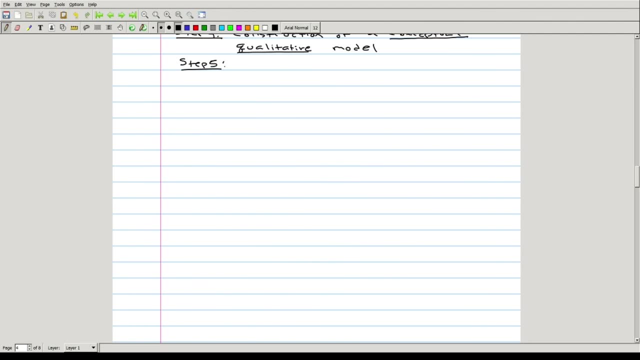 So I'm going to step back, And the last step here is conclusions making, conclusions, predictions and recommendations that follow from this qualitative model. That's the last step of this process, And these five steps are the form, the basis of a given model in science. 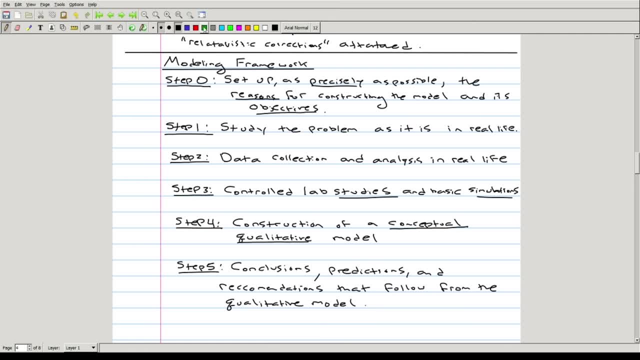 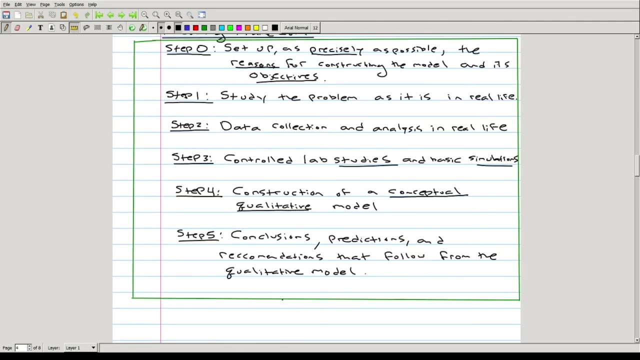 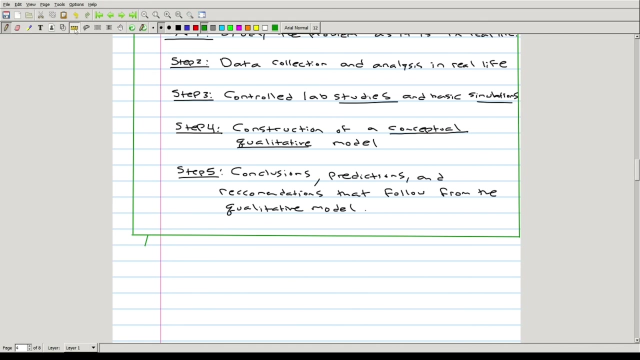 But essentially, these steps are very often not enough and these steps are only the beginning of the modeling process. So, these five steps- I've just made a box around these steps- because they all together form the basis for what's called a qualitative model. 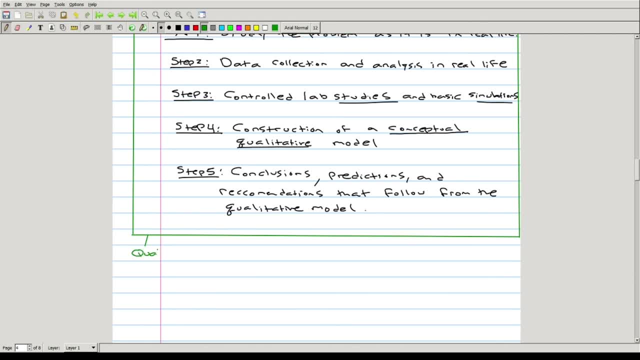 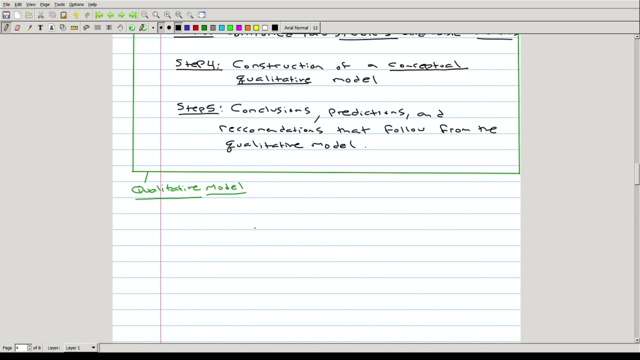 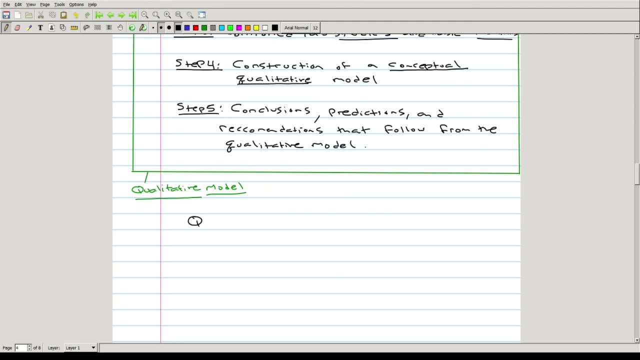 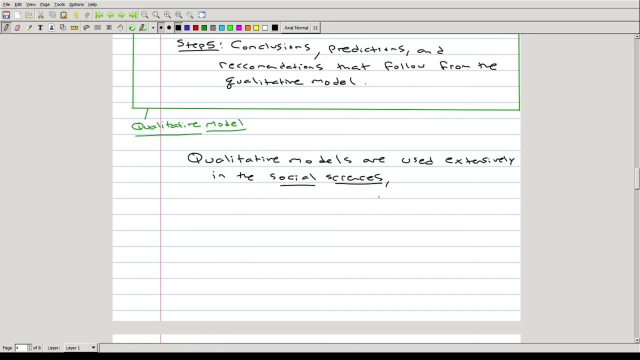 They are a standard. They are extensively used in the social sciences And they're also used in the physical sciences, the natural sciences and engineering as well. But it's important to find, it's important to point out that they are really accepted. 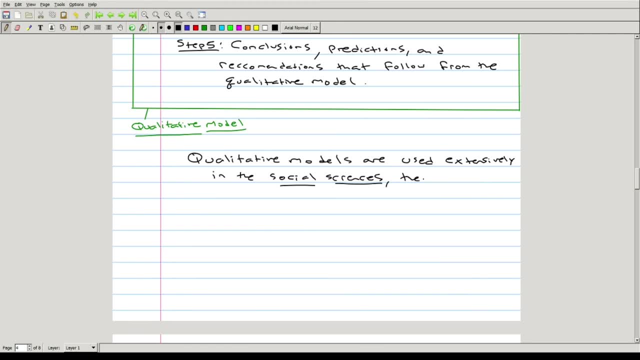 as fact in the natural sciences. And if you look at them in technology, you're going to see that these are not only the most valuable, but they're also the most valuable material. And if you look at them in technology, they are very much the most valuable material. 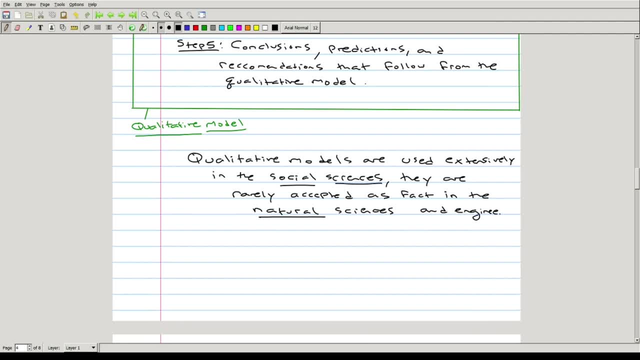 And by natural sciences. here we're talking about physics, chemistry, biology, etc. etc. In these fields we have to perform additional steps which lead to the following: to a mathematical quantitative model- And notice my use of the word quantitative here.